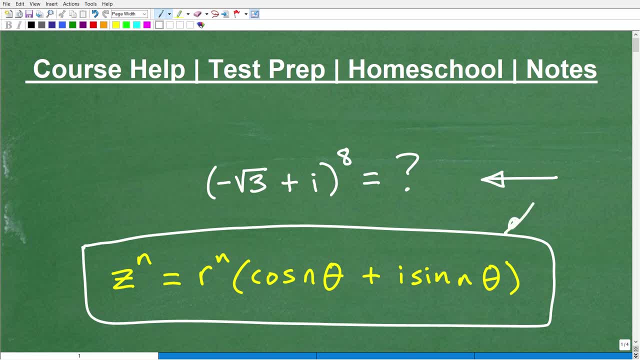 de Moore's theorem And this is kind of part of it I'm going to explain. I'm going to show you the whole theorem here in a second, But de Moore's theorem essentially allows us. it's an awesome theorem. Here is a complex number. Okay, so complex number again. remember a plus bi? Now, if I'm talking any of this stuff here and you're like totally confused and lost, well, you're probably not at this level of mathematics. But most of you should be pretty familiar with the complex number like two plus five I. this is a complex number. And then here: 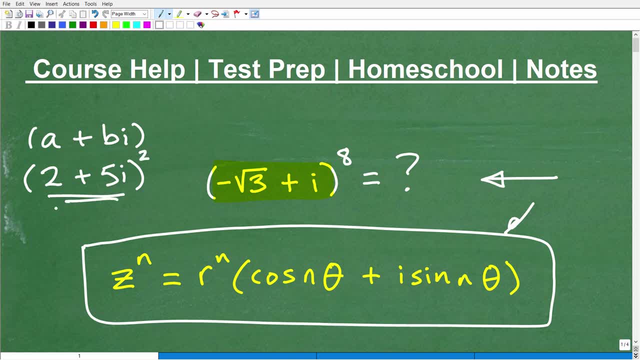 if I wanted to square this, I can just use the FOIL method and multiply this by itself and just do some basic algebra to get the answer. But if I wanted to take the eighth power of that, that means I'm going to have to take this thing and multiply it by itself eight times. that becomes a tremendous amount of work. So the de Moore's theorem allows us to take the power of complex numbers and the roots of complex numbers. And there's- I'm going to explain this, how this works. But some of you might say: well, I don't need de Moore's theorem because I'll just go ahead and do it. 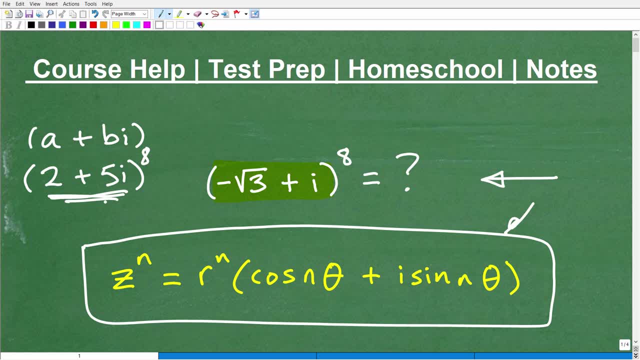 I'll just go ahead and just multiply by this thing, multiply by itself eight times. But what if I made this like 80? Okay, the 80th power of this? well then, you know most of you be like: okay, I give up, I'll learn de Moore's theorem. And that's pretty smart, Because if you're taking again this level of mathematics, you need to understand. de Moore's theorem is very, very, very important because you need to understand how to take the powers and roots of complex numbers. But we're going to focus on de Moore's theorem With this particular example. 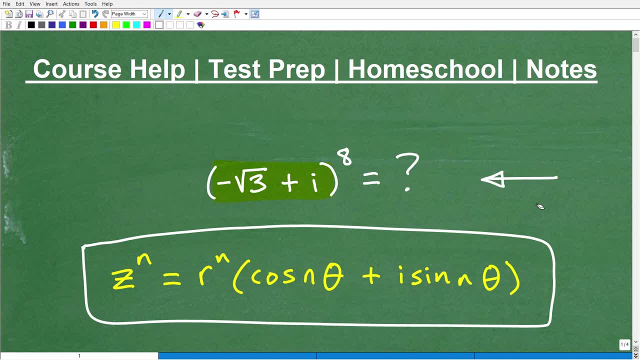 problem And I'm going to get into this step by step Now. again, if you think you think you could do this, here's a little bit of a hint: This particular problem for most people probably would take at least five minutes to do very focused work- five to even 10 minutes. So if you want to go ahead and challenge yourself- because you're learning this, you just want to see if you can get it right- Go ahead and, you know, do so. I'm going to show you the solution here in a second, But first let me quickly introduce myself. My name is john. I'm the founder of tablet class math. I'm also a 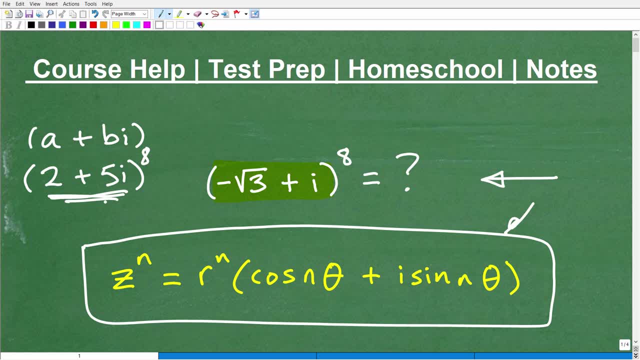 I'll just go ahead and just multiply by this thing, multiply by itself eight times. But what if I made this like 80? Okay, the 80th power of this? well then, you know most of you be like: okay, I give up, I'll learn de Moore's theorem. And that's pretty smart, Because if you're taking again this level of mathematics, you need to understand. de Moore's theorem is very, very, very important because you need to understand how to take the powers and roots of complex numbers. But we're going to focus on de Moore's theorem With this particular example. 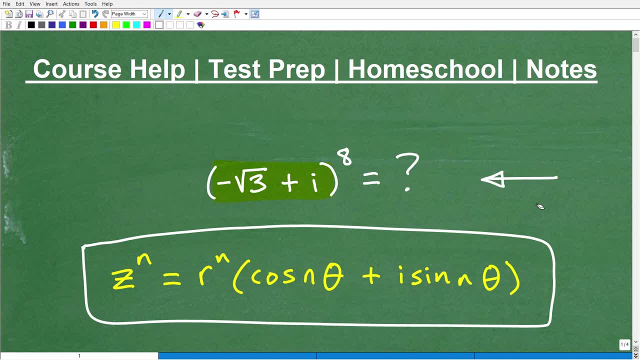 problem And I'm going to get into this step by step Now. again, if you think you think you could do this, here's a little bit of a hint: This particular problem for most people probably would take at least five minutes to do very focused work- five to even 10 minutes. So if you want to go ahead and challenge yourself- because you're learning this, you just want to see if you can get it right- Go ahead and, you know, do so. I'm going to show you the solution here in a second, But first let me quickly introduce myself. My name is john. I'm the founder of tablet class math. I'm also a 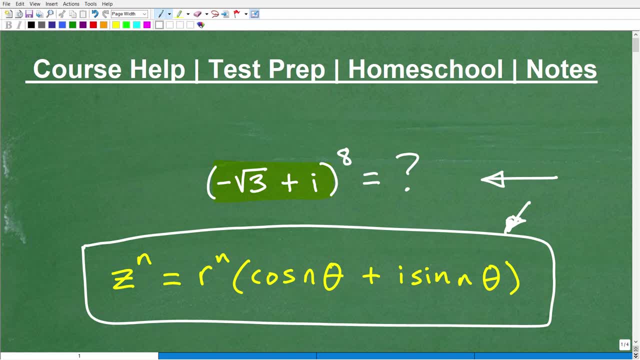 middle and high school math teacher. I'm going to leave a link to my math help program in the description of this video, But basically I have 100 plus different math courses ranging from pre algebra to pre calculus and everything in between. So if you are studying middle school, high school, even college level mathematics, I can help you pass your course. This stuff here that we're talking about de Moore's theorem- would all be in my pre calculus course For. so these for those of you out there that are possibly taking some sort of exam that has math on it, So for 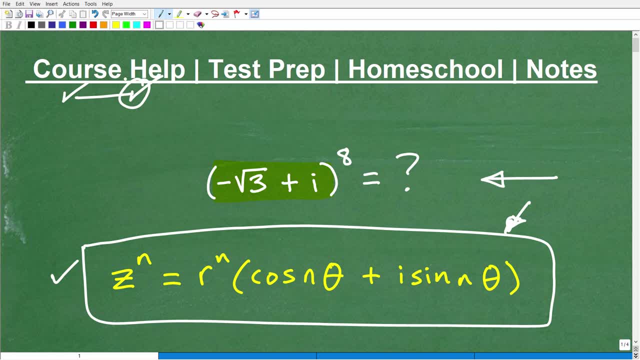 example, the GED, SAT, ACT, GRE, GMAT, ASVAB, Accuplacer, Alex exam, CLEP exam, a teacher certification exam- you get the idea. I have a ton of test prep courses that can help you prepare and pass those exams. If you homeschool, I have very comprehensive homeschool math curriculum And for those of you that don't have notes, I'm going to leave links to my notes in the description of this video. But hopefully you have great outstanding math notes. you cannot pass this level of mathematics or 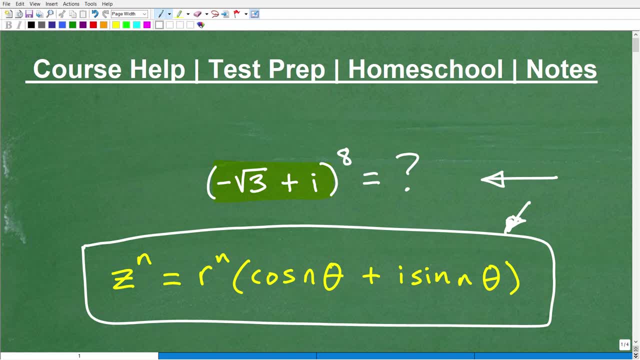 middle and high school math teacher. I'm going to leave a link to my math help program in the description of this video, But basically I have 100 plus different math courses ranging from pre algebra to pre calculus and everything in between. So if you are studying middle school, high school, even college level mathematics, I can help you pass your course. This stuff here that we're talking about de Moore's theorem- would all be in my pre calculus course For. so these for those of you out there that are possibly taking some sort of exam that has math on it, So for 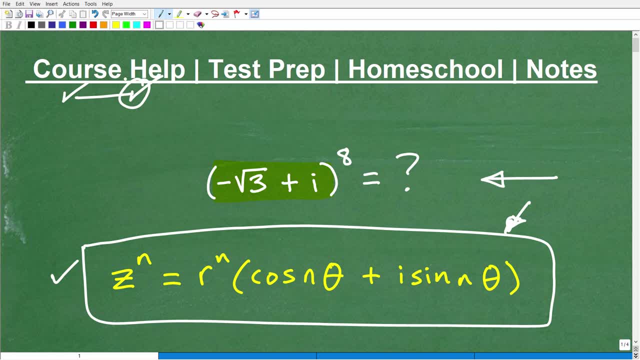 example, the GED, SAT, ACT, GRE, GMAT, ASVAB, Accuplacer, Alex exam, CLEP exam, a teacher certification exam- you get the idea. I have a ton of test prep courses that can help you prepare and pass those exams. If you homeschool, I have very comprehensive homeschool math curriculum And for those of you that don't have notes, I'm going to leave links to my notes in the description of this video. But hopefully you have great outstanding math notes. you cannot pass this level of mathematics or 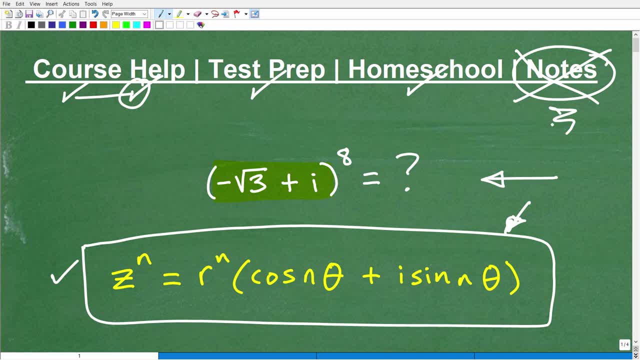 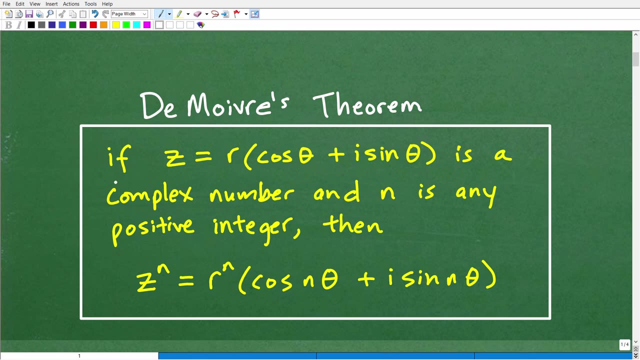 do well in any level of math without taking excellent notes. So start taking notes and everything will get a lot better. But we're going to get into de Moore's theorem right now. Okay, so let's go ahead and just review basically what de Moore's theorem is. So it says, I'll read it and I'll explain it to you. It says: if z is equal to r cosine theta plus i sine theta is a complex number and n is any positive integer, then z to the n is equal r to the n cosine n theta plus i sine theta. 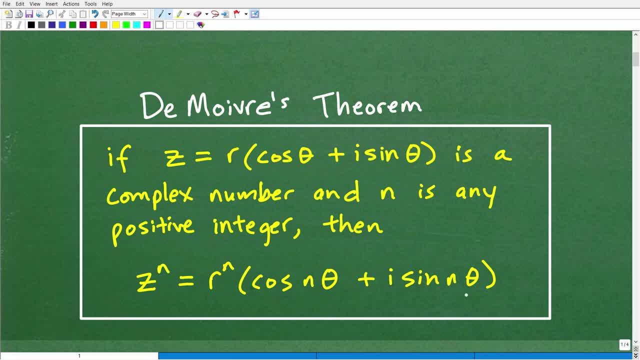 plus i, sine and theta. So if you're new to this, you know probably a lot of you are going to be like: what is this? You know this is crazy math. Well, listen again. this particular video is more targeted to those of you that are already studying this topic, But if you just like, 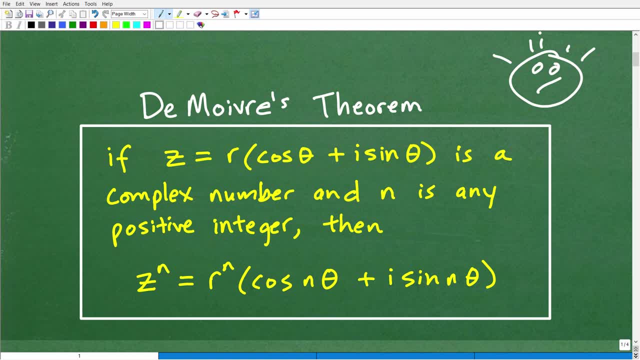 you know are interested in this, and this is the first time you're learning this. well, stick around. I think you know you'll pick up on some of the concepts here that you might be taking next. Maybe you're Algebra 2 and you just want to see a little bit. 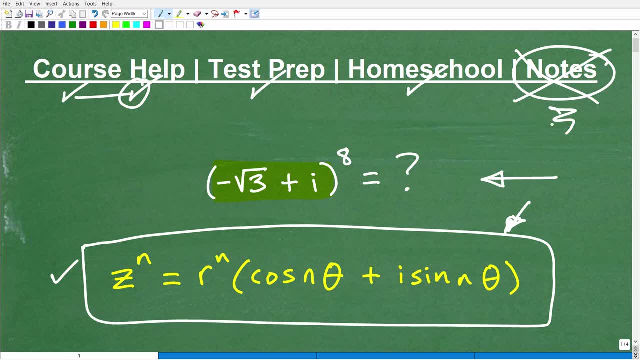 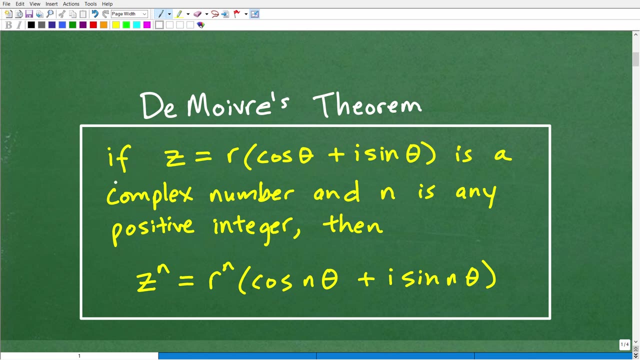 do well in any level of math without taking excellent notes. So start taking notes and everything will get a lot better. But we're going to get into De Moore's theorem right now. Okay, so let's go ahead and just review basically what De Moore's theorem is. So it says, I'll read it and I'll explain it to you. It says: if z is equal to r cos theta plus i, sine theta is a complex number and n is any positive integer, then z to the n is equal r to the n cos n theta and n is any positive integer, then z to the n is equal r to the n cos n theta and n is any positive integer. 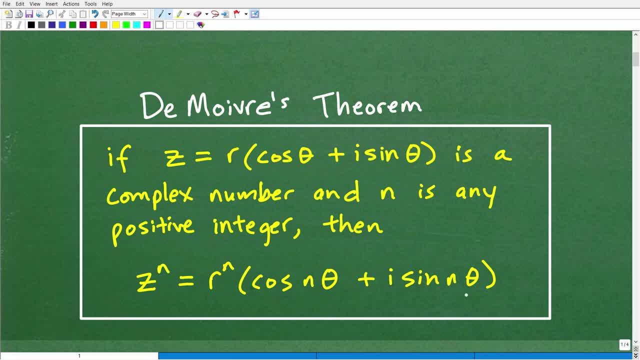 plus i, sine and theta. So if you're new to this, you know probably a lot of you are going to be like: what is this? You know this is crazy math. Well, listen again. this particular video is more targeted to those of you that are already studying this topic, But if you just like, 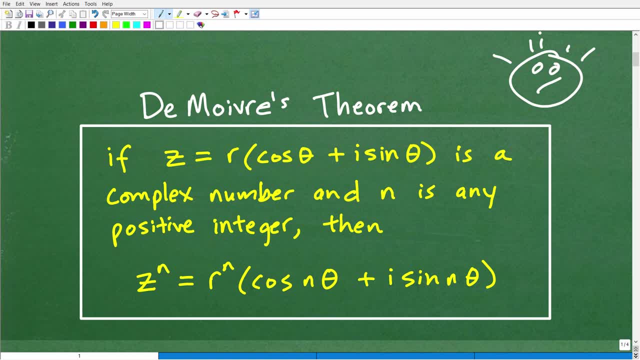 you know are interested in this, and this is the first time you're learning this. well, stick around. I think you know you'll pick up on some of the concepts here that you might be taking next. Maybe you're Algebra 2 and you just want to see a little bit. 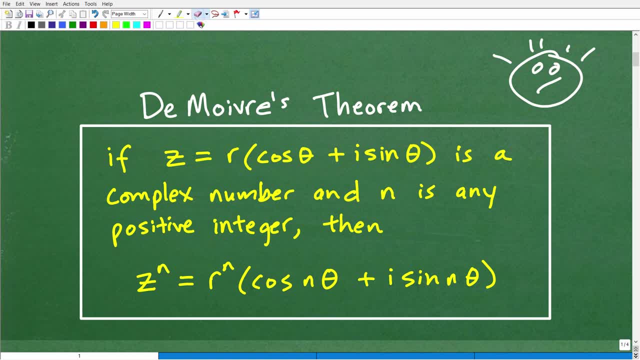 of the math that's right around the corner. All right, So what are we talking about here, Okay? Well, here's the thing. Z, okay, represents some sort of complex number. So let's say Z is our complex number, like this: 2 plus 3i. But this complex number is an a plus bi form. Okay, We call. 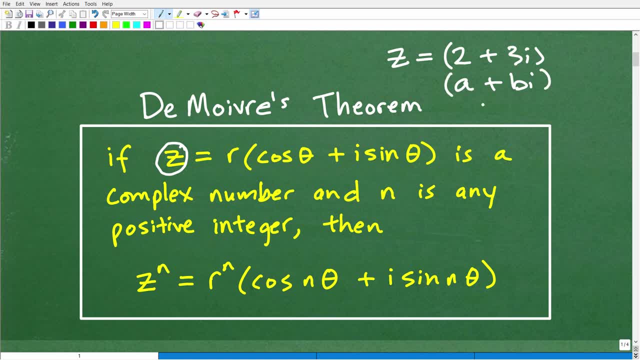 this kind of standard or rectangular form. So we can't use DeMorphe's theorem when a complex number is a complex number. So we can't use DeMorphe's theorem when a complex number is a complex number. So we can't use DeMorphe's theorem when a complex number is a complex number. So we can't use. 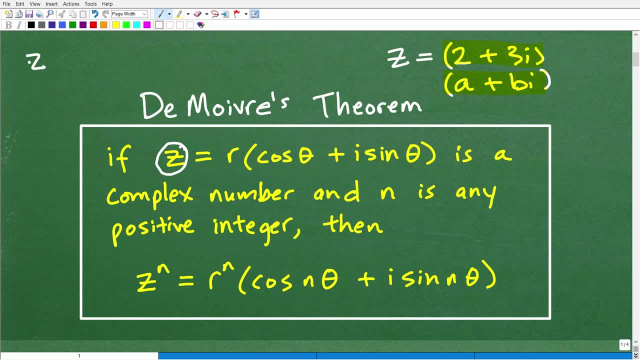 DeMorphe's theorem when a complex number is written in this form. Okay, So we have this complex number. Let's take this particular complex number as an example: 2 plus 3i. What we need to do is to write this into what we call trigonometric or polar form. Okay, This. 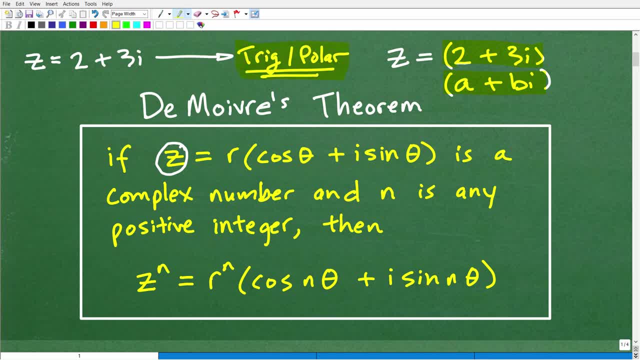 right here is a pretty involved process in and of itself. Okay, And this is the thing I'm not going to get into and cover, You need to know, in order to do DeMorphe's theorem, you need to know how to take complex numbers and write them into trigonometric and polar form. So 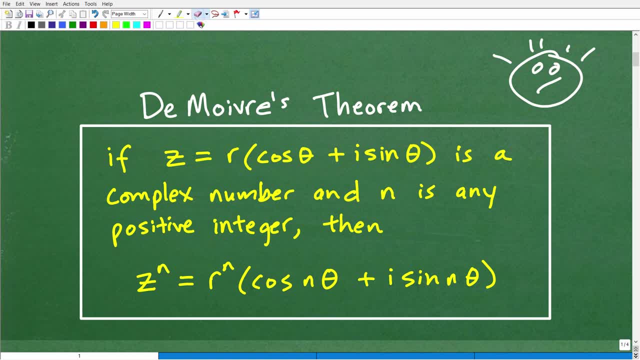 of the math that's right around the corner. All right, So what are we talking about here, Okay? Well, here's the thing. Z, okay, represents some sort of complex number. So let's say Z is our complex number, like this: 2 plus 3i. But this complex number is an a plus bi form. Okay, We call. 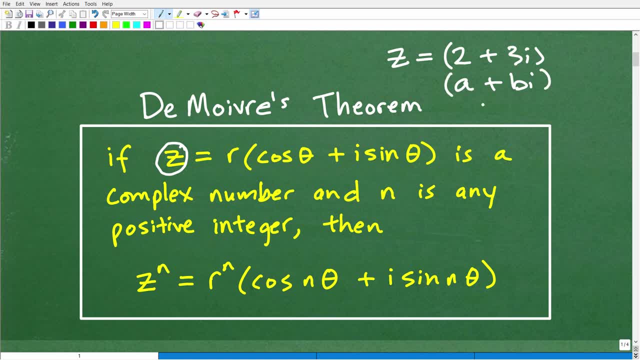 this kind of standard or rectangular form. So we can't use DeMorphe's theorem when a complex number is a complex number. So we can't use DeMorphe's theorem when a complex number is a complex number. So we can't use DeMorphe's theorem when a complex number is a complex number. So we can't use. 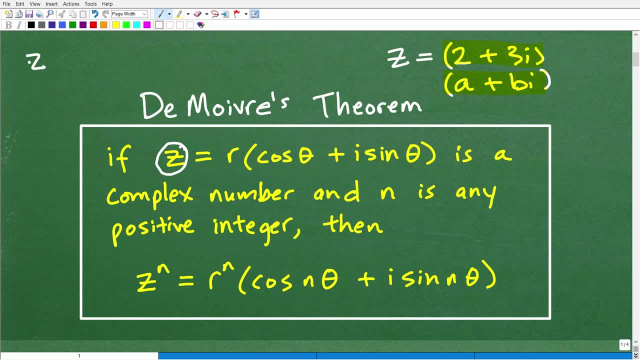 DeMorphe's theorem when a complex number is written in this form. Okay, So we have this complex number. Let's take this particular complex number as an example: 2 plus 3i. What we need to do is to write this into what we call trigonometric or polar form. Okay, This. 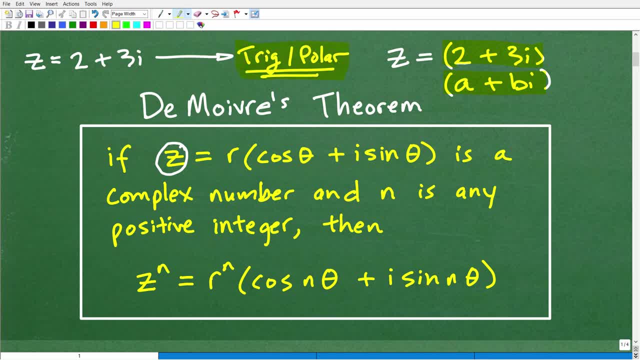 right here is a pretty involved process in and of itself. Okay, And this is the thing I'm not going to get into and cover, You need to know, in order to do DeMorphe's theorem, you need to know how to take complex numbers and write them into trigonometric and polar form. So 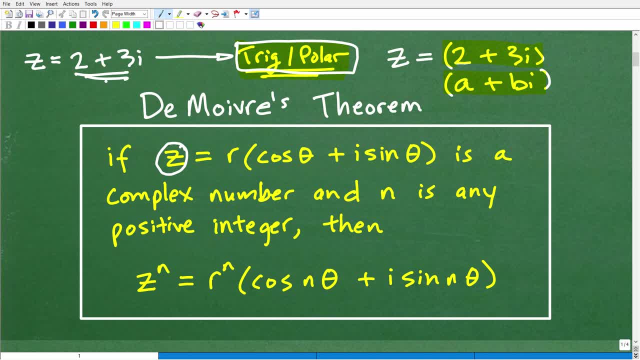 if this is the part of the theorem that's troubling you, then I'll try to do some additional videos on some example problems, But I would strongly suggest that you check out my pre-calculus course, because I get into all this really thoroughly. Okay, And this can be complicated and confusing. 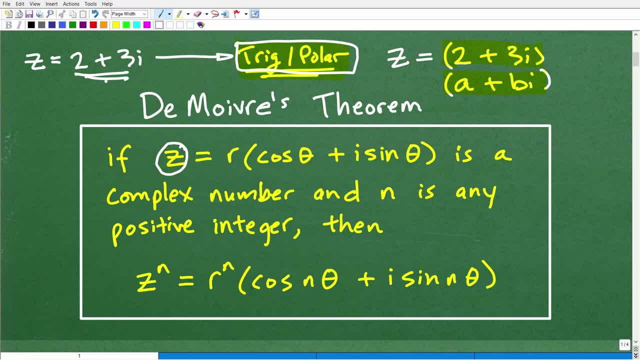 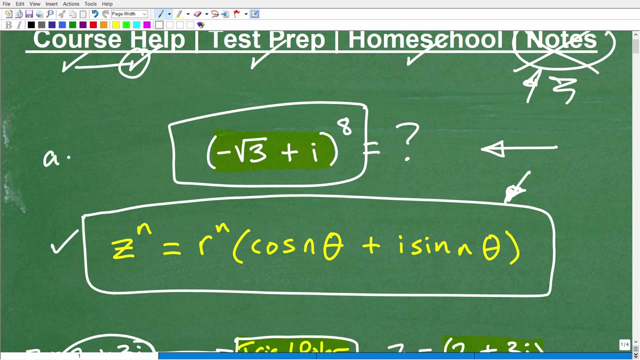 especially when you're asked to do these problems without a calculator. So first things first. if we have a complex number that's not in trigonometric form, like this particular example, let me just go up here real quick. Here, this is not in polar or trigonometric form, This is in rectangular or a plus bi form. So I can't do. 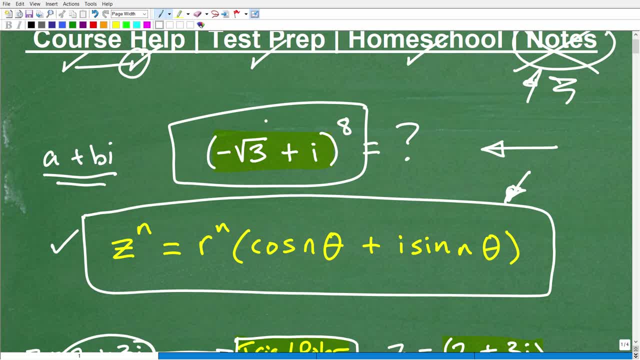 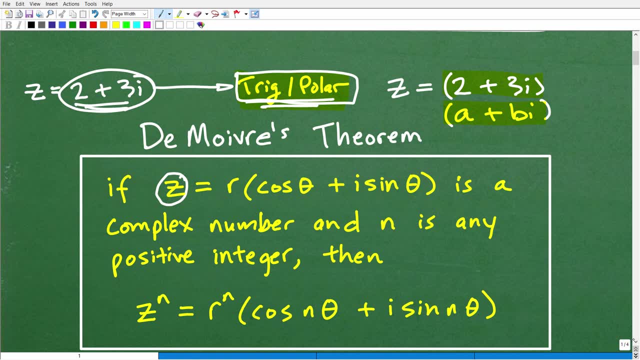 this problem. yet I can't take the eighth power of this complex number z, until I put this into trigonometric or polar form. So again, you should have your math notes And if you want to, you know, pause the video and go ahead and see if you can do that, then you know pursue. 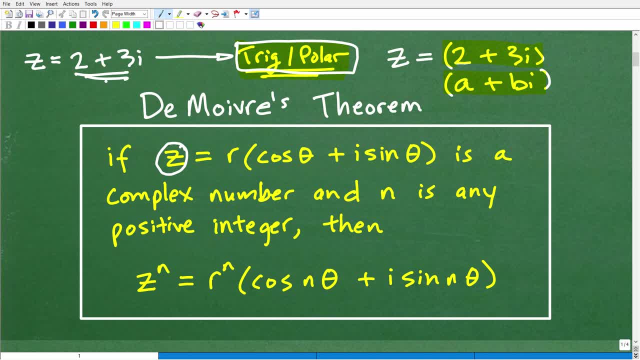 if this is the part of the theorem that's troubling you, then I'll try to do some additional videos on some example problems, But I would strongly suggest that you check out my pre-calculus course, because I get into all this really thoroughly. Okay, And this can be complicated and confusing. 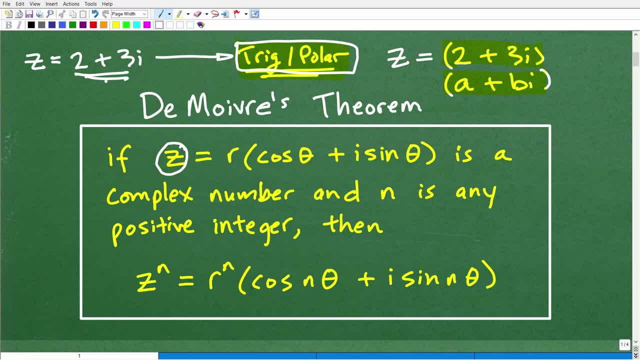 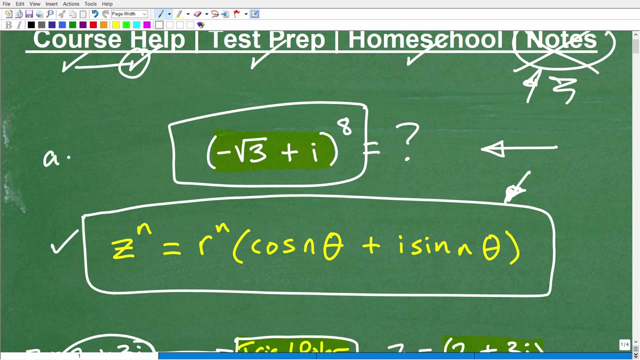 especially when you're asked to do these problems without a calculator. So first things first. if we have a complex number that's not in trigonometric form, like this particular example, let me just go up here real quick. Here, this is not in polar or trigonometric form, This is in rectangular or a plus bi form. So I can't do. 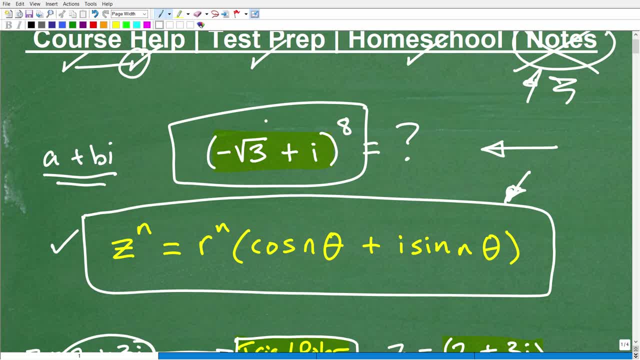 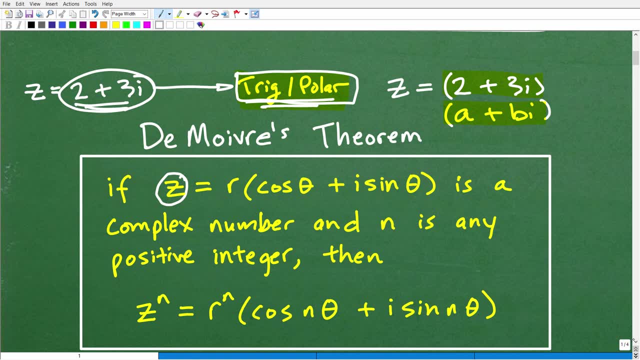 this problem. yet I can't take the eighth power of this complex number z, until I put this into trigonometric or polar form. So again, you should have your math notes And if you want to, you know, pause the video and go ahead and see if you can do that, then you know pursue. 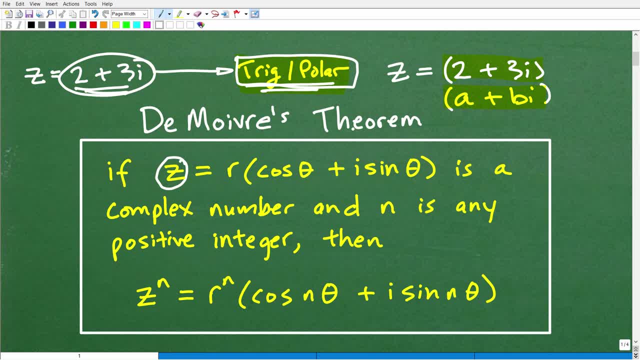 You know, see if you can get the right answer. So the bottom line with de Morve's theorem here is that z, our complex number, has to be in trigonometric form, And that's r cosine theta plus i sine theta, Or sometimes it's r cis. Well, it's all the same thing, But this should be. 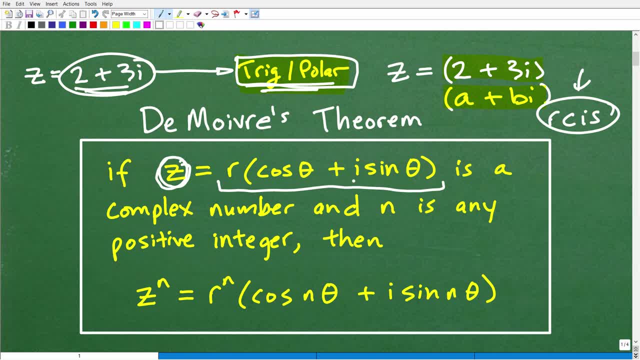 familiar to you if you expect to understand de Morve's theorem. Okay, So once we have this complex number and it's expressed in trigonometric or polar form, then we just go ahead and follow This formula right here. okay, our complex number to the nth power. So here, in this particular 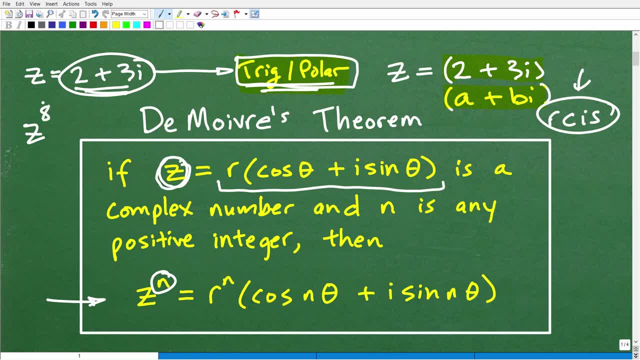 problem. we have some sort of complex number And we're going to be taking it to the eighth power, And so we would just go ahead and plug in the respective values into this particular formula. Okay, So let's go ahead and get to it. That is de Morve's theorem. Again, if this is the first time, 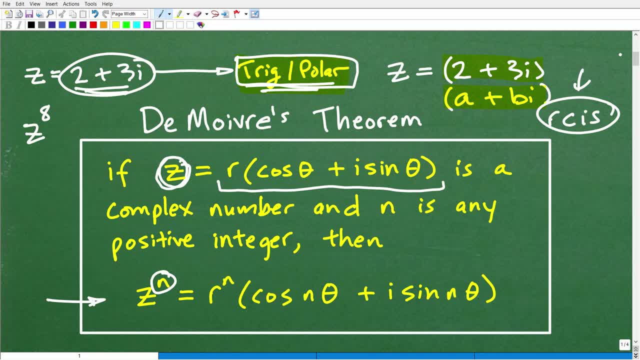 you're trying to understand de Morve's theorem. this is probably not going to cut it as a full comprehensive lesson Again, at least not until you get to the nth power. So let's go ahead. and as far as my teaching goes, you might want to check out my pre-calculus course. But let's get. 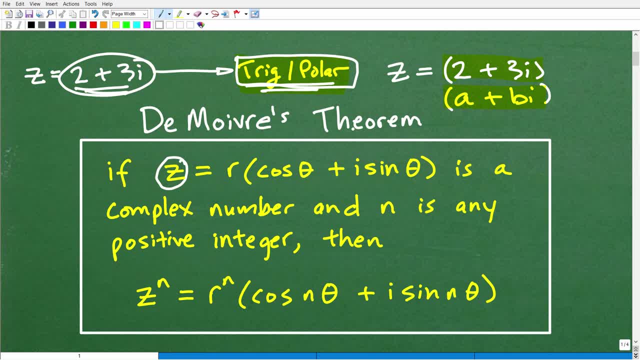 You know, see if you can get the right answer. So the bottom line with de Morve's theorem here is that z, our complex number, has to be in trigonometric form, And that's r cosine theta plus i sine theta, Or sometimes it's r cis. Well, it's all the same thing, But this should be. 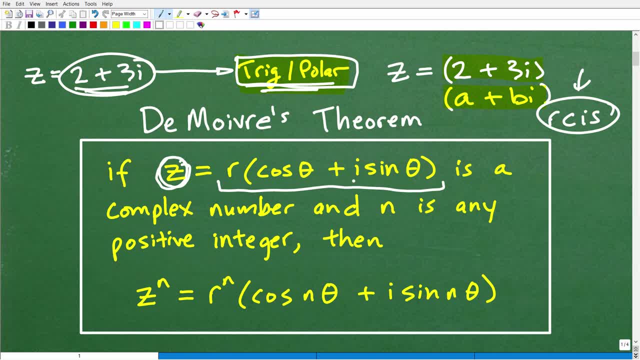 familiar to you if you expect to understand de Morve's theorem. Okay, So once we have this complex number and it's expressed in trigonometric or polar form, then we just go ahead and follow This formula right here. okay, our complex number to the nth power. So here, in this particular 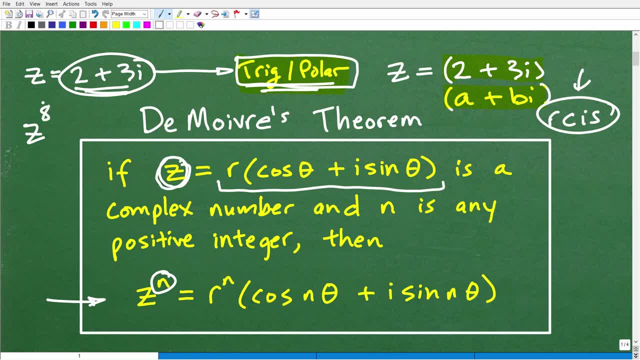 problem. we have some sort of complex number And we're going to be taking it to the eighth power, And so we would just go ahead and plug in the respective values into this particular formula. Okay, So let's go ahead and get to it. That is de Morve's theorem. Again, if this is the first time, 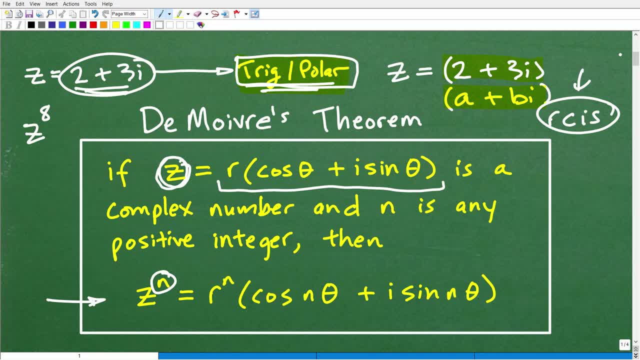 you're trying to understand de Morve's theorem. this is probably not going to cut it as a full comprehensive lesson Again, at least not until you get to the nth power. So let's go ahead. and as far as my teaching goes, you might want to check out my pre-calculus course. But let's get. 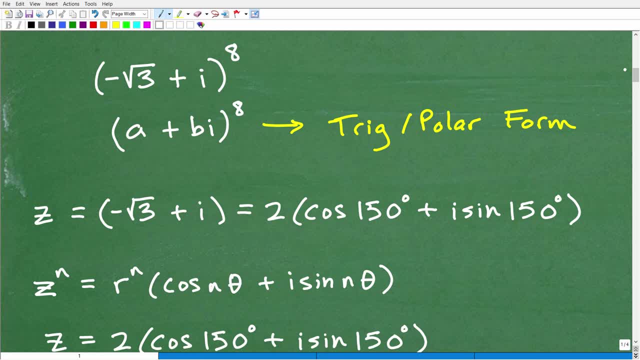 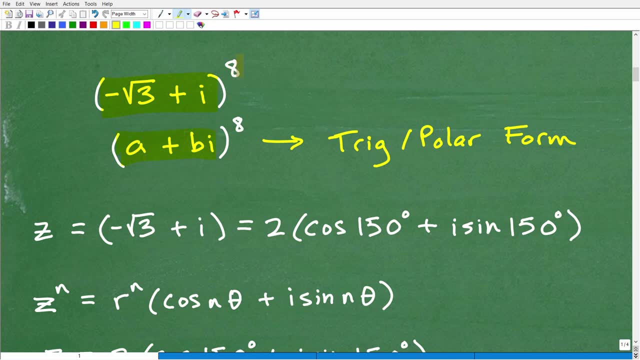 to the actual problem. All right. So here is the problem. Here's our complex number. It's an, a plus bi form, Okay, Rectangular form. But I want to take this complex number to the eighth power. Okay, Well, first things first. I need to express this into trigonometric or polar form, All right, 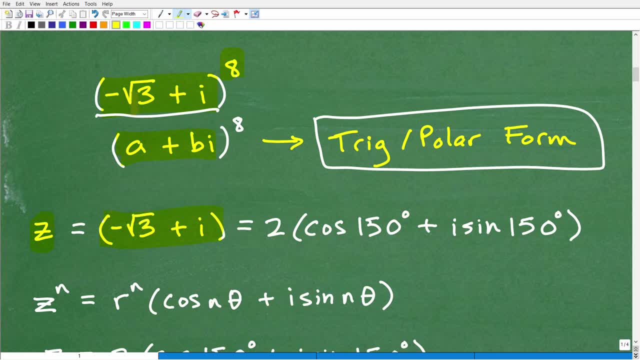 So our complex number z- and here it is right here- which is three plus i, is equal to two times cosine 150 degrees plus i sine 150 degrees. This right here, this complex number, this is the equivalent, This is the complex number expressed. 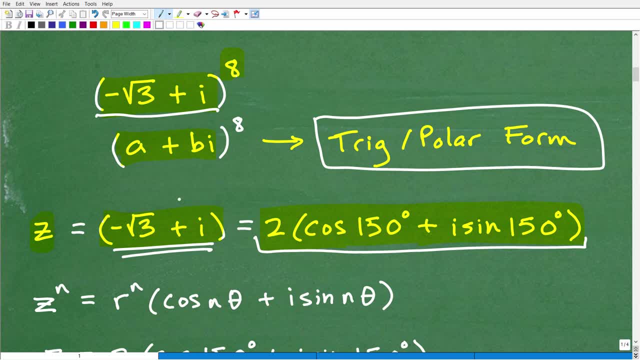 in trigonometric or polar form. Okay. So to go from here to here is a whole lesson in and of itself. So if you don't know how to do this, a lot of students struggle with this part of it. They can't, you know. they struggle with taking a. 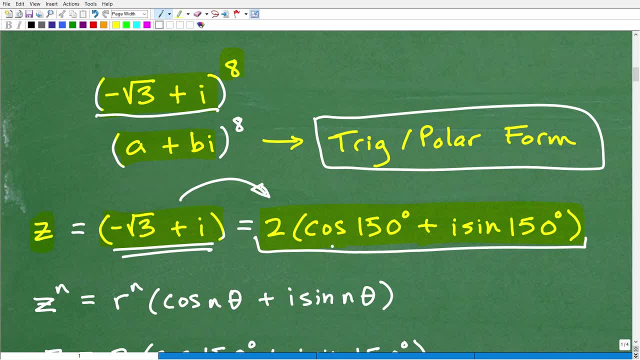 a complex number that's in a rectangular form and putting it in to a polar form. If you can't do that, well then it's. you know it's game over in terms of solving this problem, because we have to have this complex number written or expressed in this way, And of course I'm using degrees. 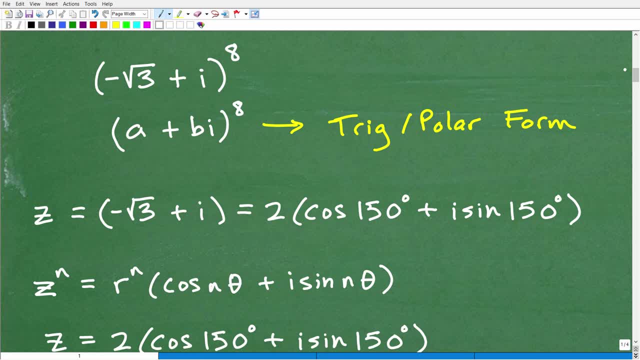 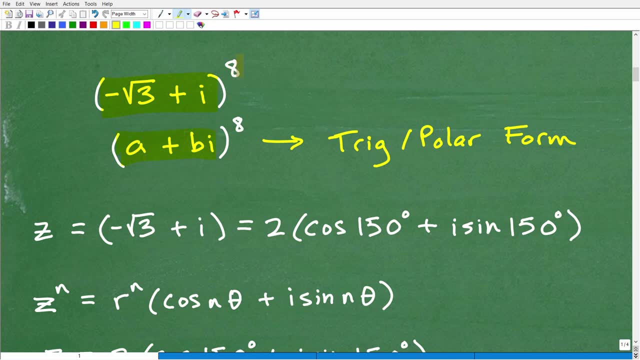 to the actual problem. All right. So here is the problem. Here's our complex number. It's an, a plus bi form, Okay, Rectangular form. But I want to take this complex number to the eighth power. Okay, Well, first things first. I need to express this into trigonometric or polar form, All right, 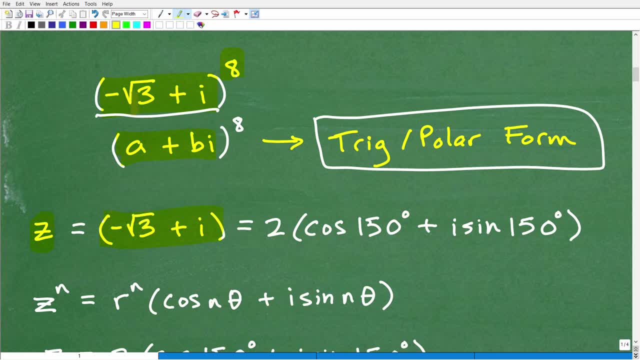 So our complex number z- and here it is right here- which is three plus i, is equal to two times cosine 150 degrees plus i sine 150 degrees. This right here, this complex number, this is the equivalent, This is the complex number expressed. 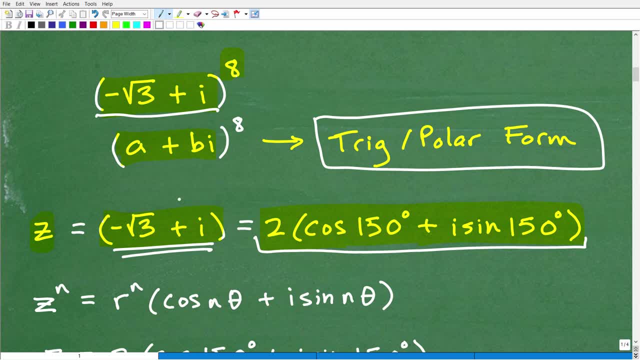 in trigonometric or polar form. Okay. So to go from here to here is a whole lesson in and of itself. So if you don't know how to do this, a lot of students struggle with this part of it. They can't, you know. they struggle with taking a. 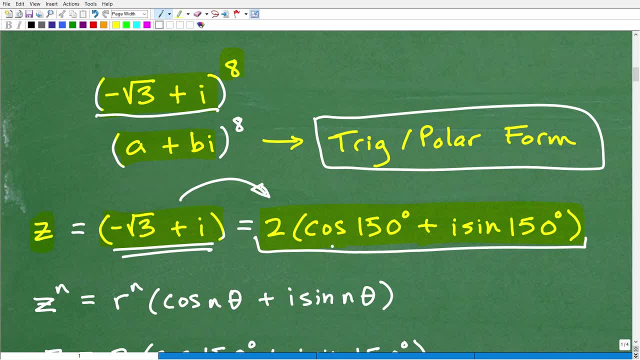 a complex number that's in a rectangular form and putting it in to a polar form. If you can't do that, well then it's. you know it's game over in terms of solving this problem, because we have to have this complex number written or expressed in this way, And of course I'm using degrees. 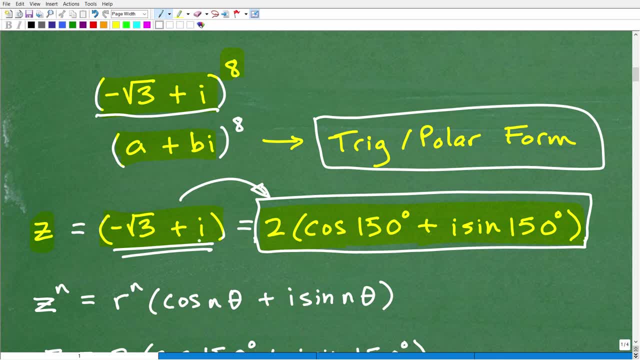 not radians, but sometimes you, you, you certainly could use radians to express your degrees, Okay. So again, I'm not showing you the steps here to do this. That's a whole. you know that this requires. you know you have to be able to do this, So I'm not showing you the steps here to do this. 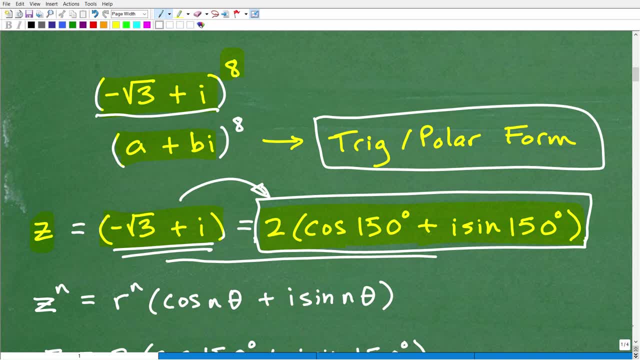 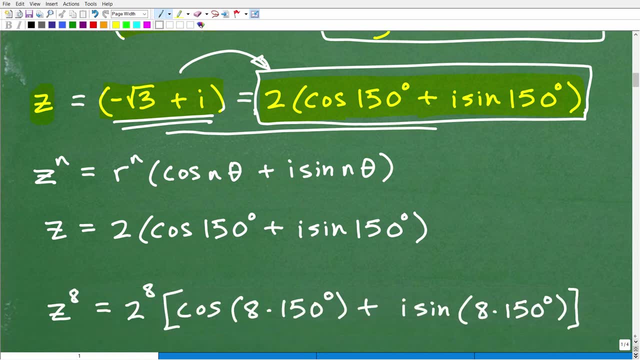 There's a decent amount of- well, not too much amount of work, but a decent amount of work to go from here to here. Just know that this is the case, All right. So let's take it up from this point. So our complex number Z, if we take it to some power, we're going to be taking this particular 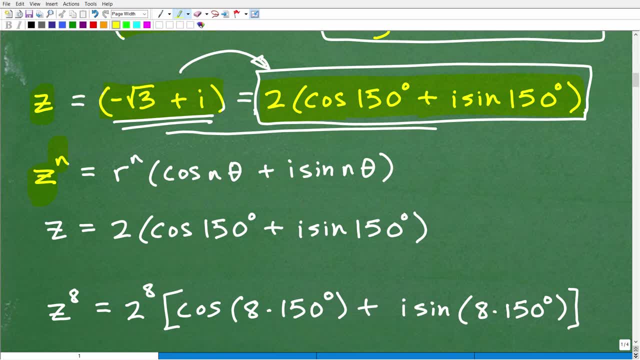 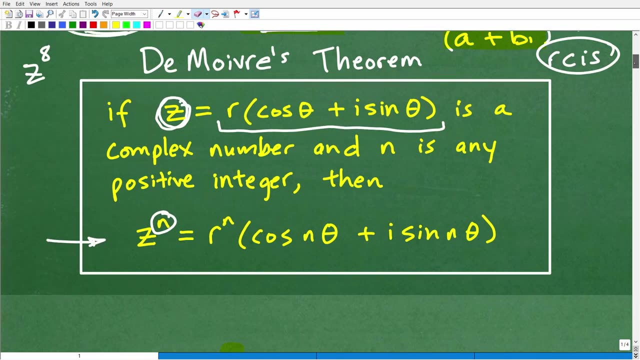 complex number to the eighth power. Okay, Whatever it is, though, our complex number Z to the nth power is R, which is the radius. Okay, In this case, that's two. All right, right here, When you have a complex number, let me just go back here. All right? So let's review and 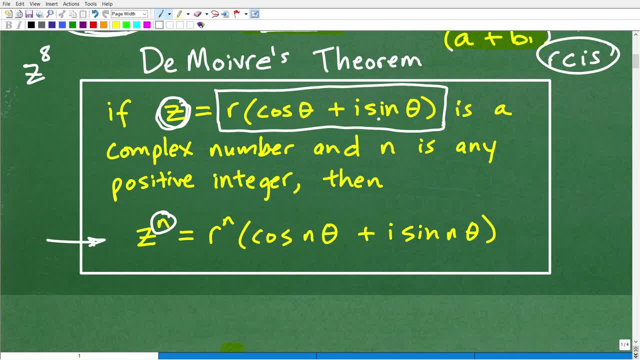 DeMores. theorem R: cosine theta plus I sine theta. This is the radius, This is the angle. Again, if this is all confusing for you- you don't even know what this means- then you're not going to understand what we're talking about here. But I just want to make sure that you. 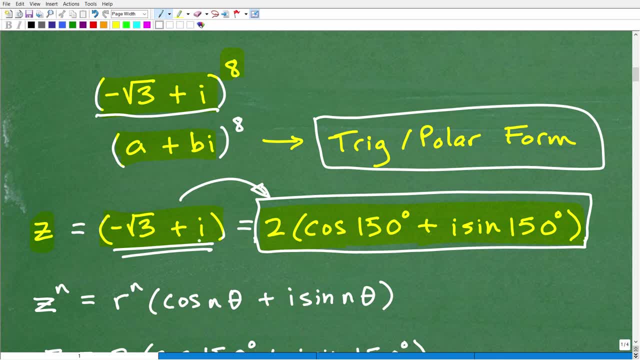 not radians, but sometimes you, you, you certainly could use radians to express your degrees, Okay. So again, I'm not showing you the steps here to do this. That's a whole. you know that this requires. you know you have to be able to do this, So I'm not showing you the steps here to do this. 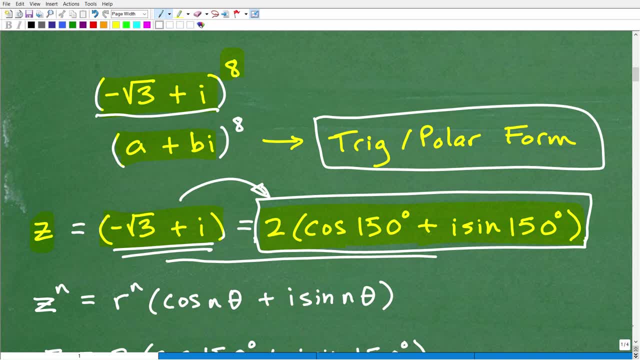 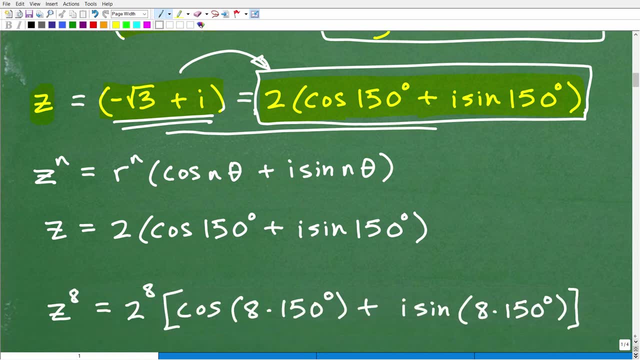 There's a decent amount of- well, not too much amount of work, but a decent amount of work to go from here to here. Just know that this is the case, All right. So let's take it up from this point. So our complex number Z, if we take it to some power, we're going to be taking this particular 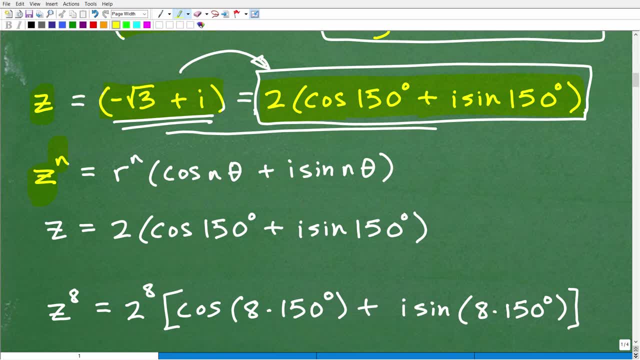 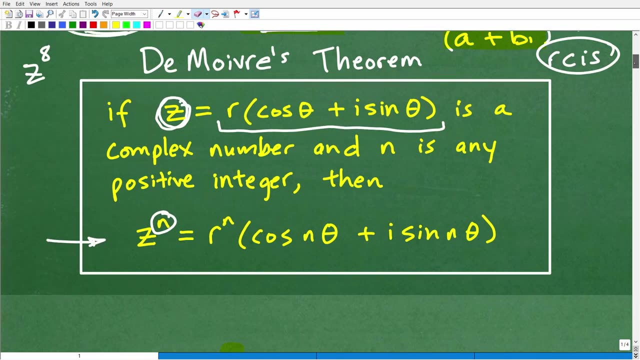 complex number to the eighth power. Okay, Whatever it is, though, our complex number Z to the nth power is R, which is the radius. Okay, In this case, that's two. All right, right here, When you have a complex number, let me just go back here. All right? So let's review and 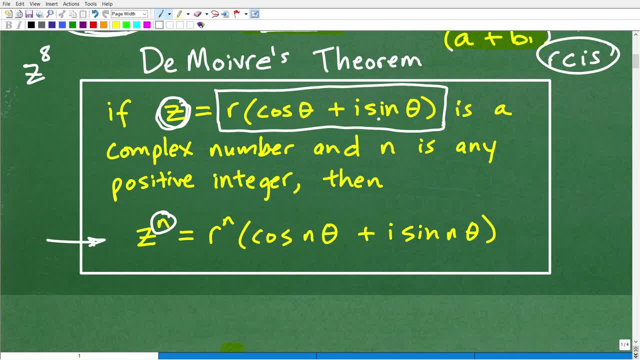 DeMorse theorem: R cosine theta plus I sine theta. This is the radius, This is the angle. Again, if this is all confusing for you- you don't even know what this means- then you're not going to understand what we're talking about here. But I just want to make sure that you. 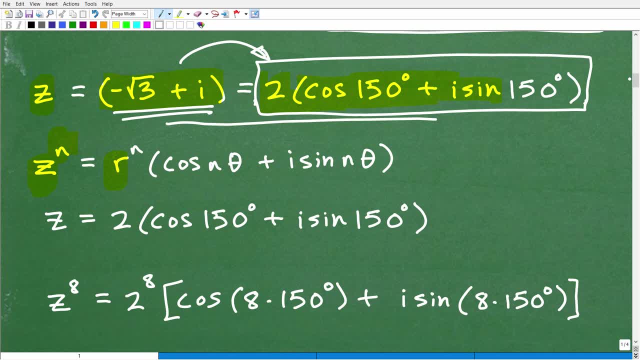 you know, are you know being able to stay with me as I explain this problem? All right, So R to the nth power. in this case that's going to be two Cosine, okay. n is our power In this. 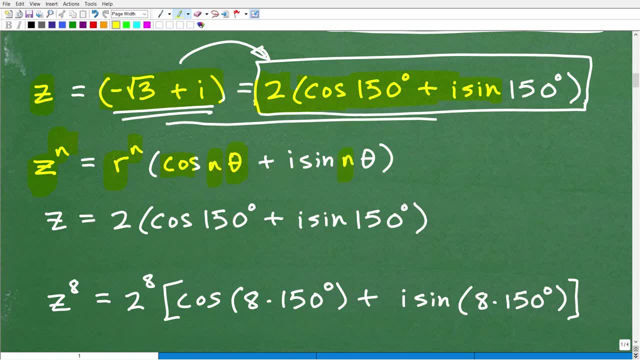 case it's going to be eight times the angle plus I, sine n times the angle. All right, So let's go ahead and get to it. Here's our complex number, Z. Okay, We already discussed that. Here it is. This is the number expressed in trigonometric form, So that's two cosine 150 degrees plus I. 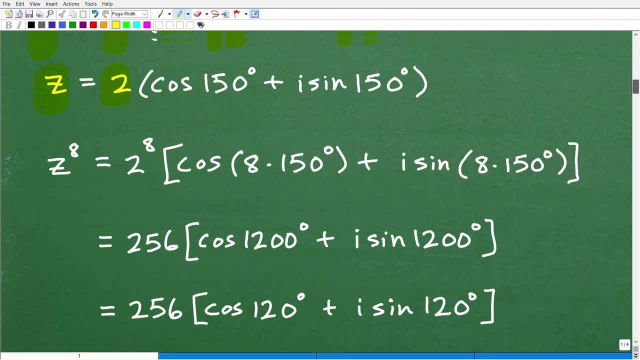 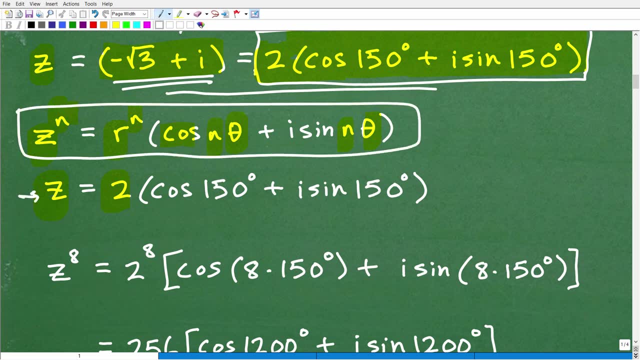 sine 150 degrees. Okay, So now let's go ahead and apply DeMorse Theorem. So this is DeMorse theorem. Here's our complex number, Z. We're just going to basically follow the you know formula here. So Z, our complex number to the eighth power, is two to the 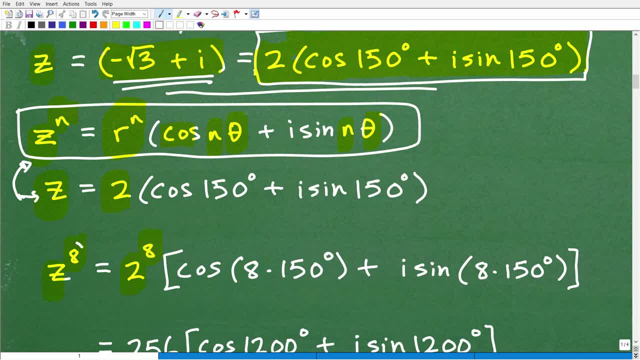 eighth, That's R to the n. Okay, Remember n, this is n, whatever power we're taking it to. Okay, That is a positive integer. So eight, here is n for this particular prompt. So that's two to the eighth power. 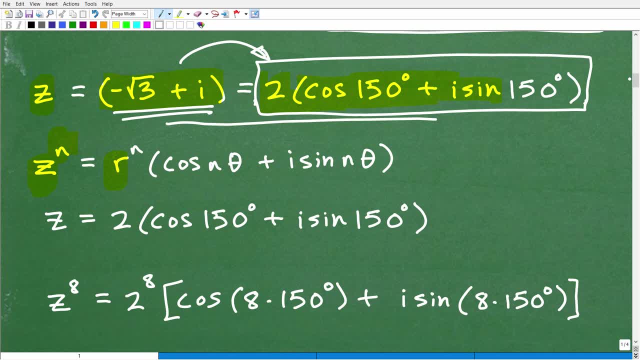 you know, are you know being able to stay with me as I explain this problem? All right, So R to the nth power. in this case that's going to be two Cosine, okay. n is our power In this. 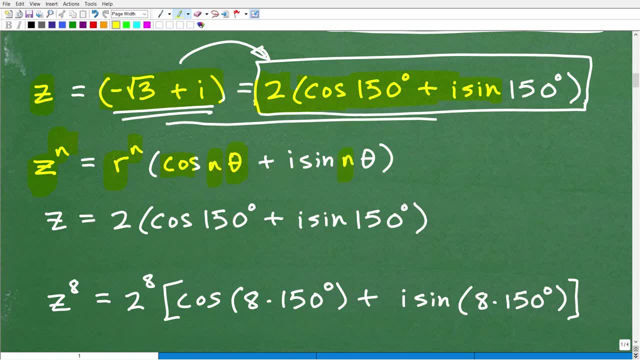 case it's going to be eight times the angle plus I, sine n times the angle. All right, So let's go ahead and get to it. Here's our complex number, Z. Okay, We already discussed that. Here it is. This is the number expressed in trigonometric form, So that's two cosine 150 degrees plus I. 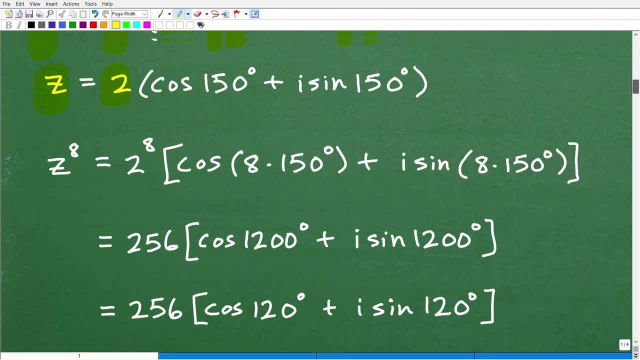 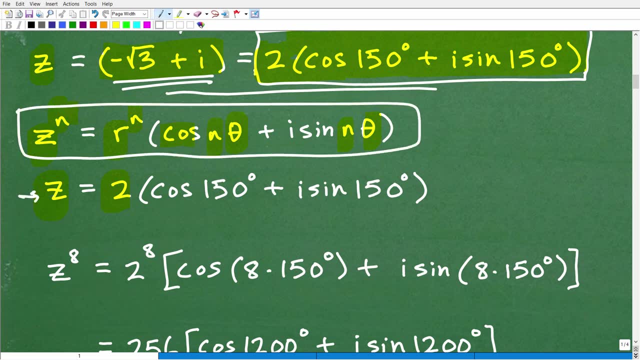 sine 150 degrees. Okay, So now let's go ahead and apply DeMores Theorem. So this is DeMores theorem. Here's our complex number, Z. We're just going to basically follow the you know formula here. So Z, our complex number to the eighth power, is two to the. 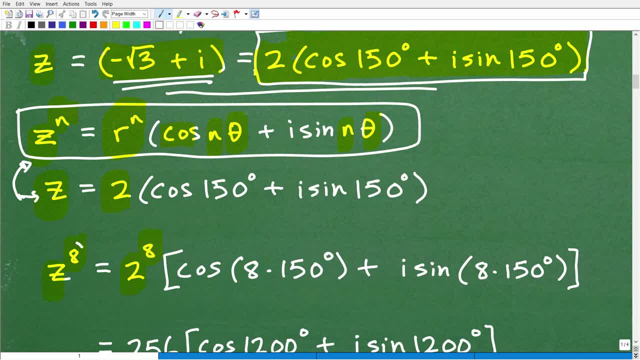 eighth, That's R to the n. Okay, Remember n, this is n, whatever power we're taking it to. Okay, That is a positive integer. So eight, here is n for this particular prompt. So that's two to the eighth power. 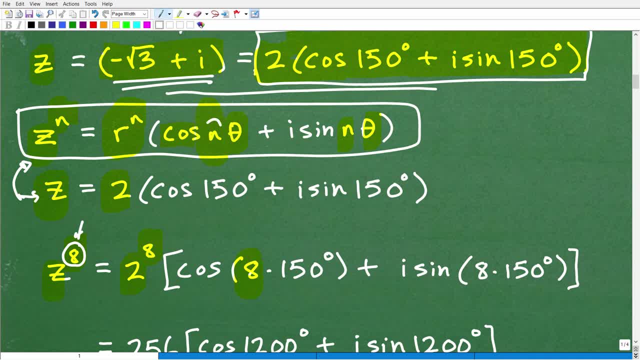 Cosine n. Okay, Remember, this is DeMores theorem- n times the angle, So that's going to be eight times 150 degrees. eight times 150 plus I sine n, which is again um eight times 150 degrees. 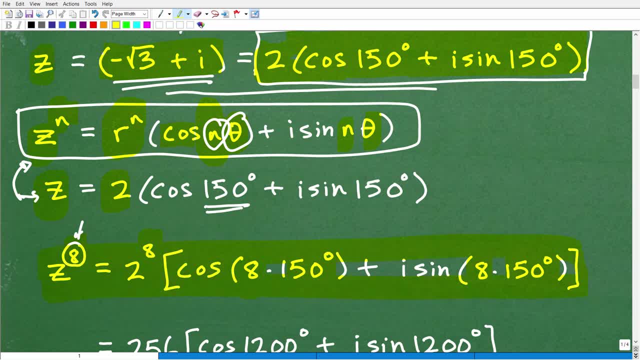 So here is the setup, Okay. So if you understand this, then that's excellent. Um, at least you got the setup correctly. but this is a good amount of work just to get to this point right. We had to go. we had to take the complex number put into trigonometric form. 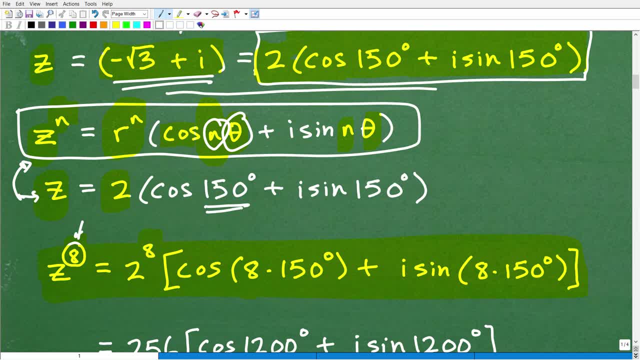 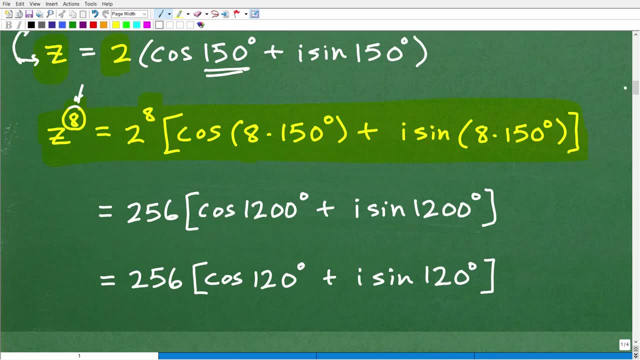 And then we had to plug it in to DeMores theorem. Now we're about ready to start the rest of the problem. Now this particular problem. um, for those of you who are taking, let's say, pre-calculus, your teacher can easily say: do this problem without the aid of a calculator. If you were in, 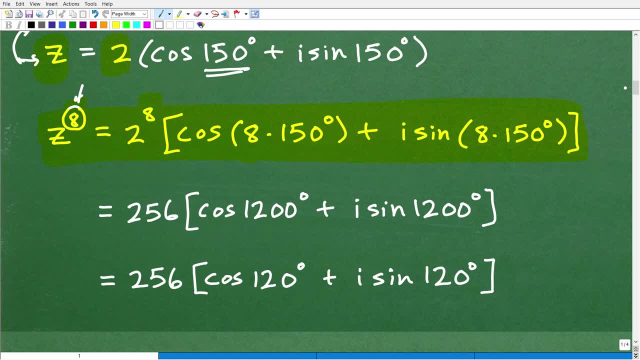 my course I'd say: put your calculator away, Show me what you know about trigonometry up to this point. But sometimes you'll- um, you'll have to do problems with your calculator or without your calculator. But this particular one would be a problem that you could do without your calculator. 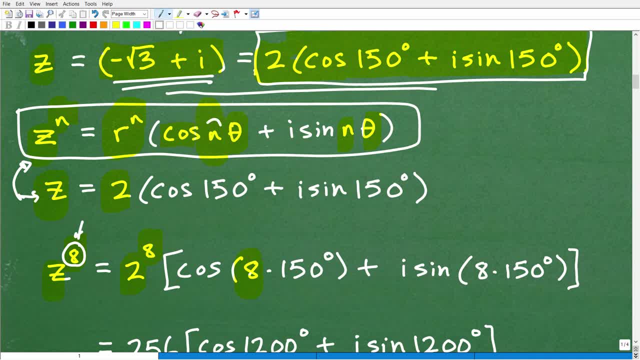 Cosine n. Okay, Remember, this is DeMorse theorem. n times the angle, So that's going to be eight times 150 degrees. eight times 150 plus I sine n, which is again eight times 150 degrees. So here: 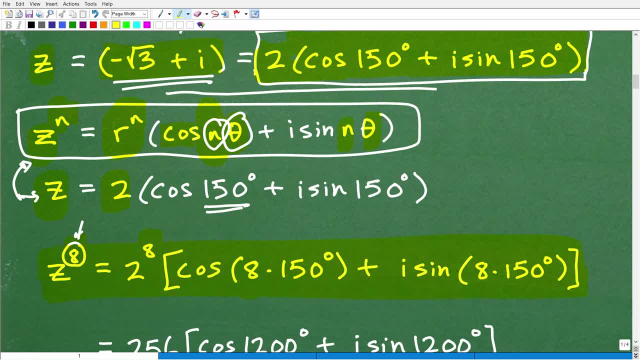 is the setup Okay. So if you understand this, then that's excellent. At least you got the setup correctly. but this is a good amount of work. just to get to this point right, We had to go. we had to take the complex number put into trigonometric form. 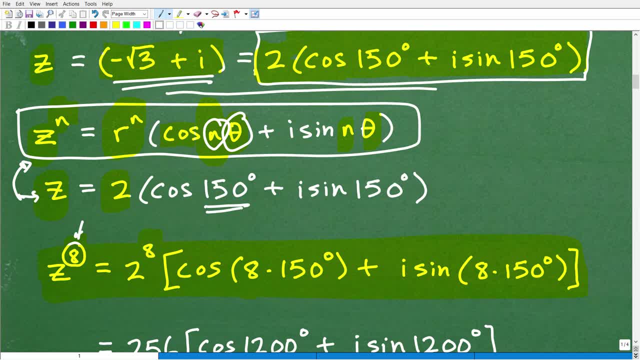 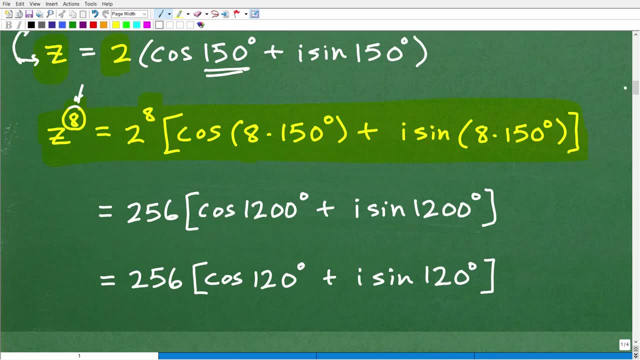 and then we had to plug it in to DeMorse theorem. Now we're about ready to start the rest of the problem. Now this particular problem for those of you who are taking, let's say, pre-calculus. your teacher can easily say: do this problem without the aid of a calculator. If you were in, 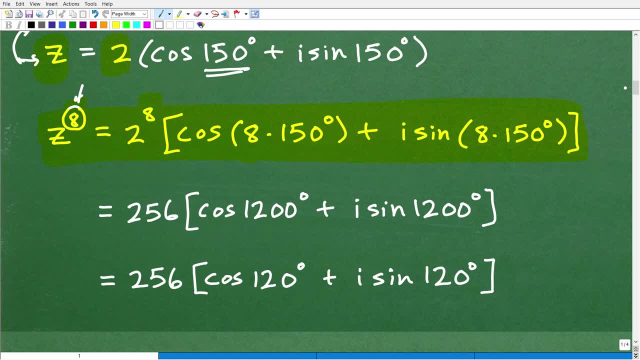 my course I'd say: put your calculator away, show me what you know about trigonometry up to this point. But sometimes you'll have to do problems with your calculator or without your calculator. But this particular one would be a problem that you could do without your calculator. 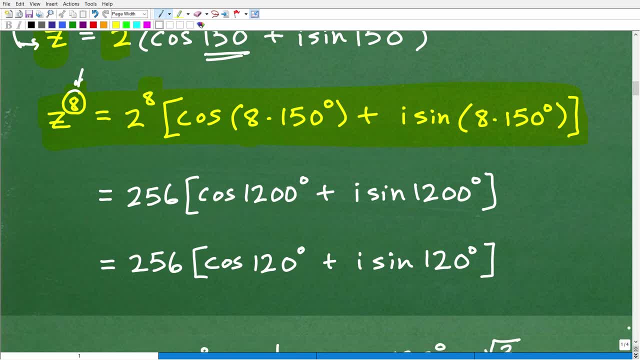 So again, you know it's a lot of work, All right, So let's go ahead and do the actual work here. Okay, The number crunching So two to the eighth is 256,. cosine eight times 150 degrees, That's. 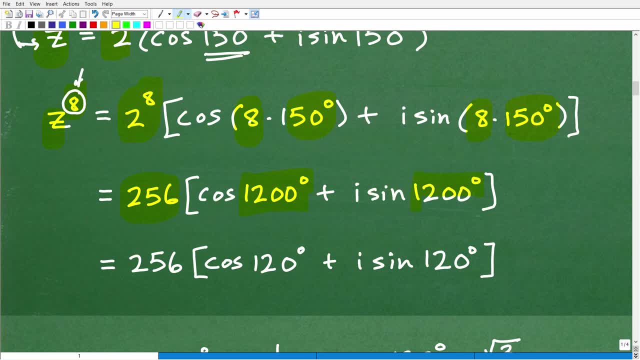 1200 degrees. I sine eight times 150, 1200 degrees. Okay, So 1200 degrees. if you looked at the unit circle, that's 360, that's 720, it's going round and round. You would end up with a. 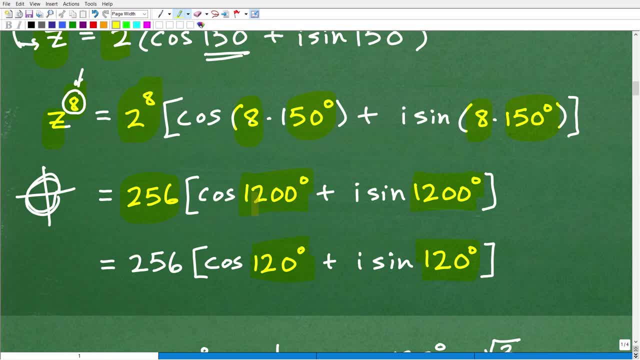 120 degrees as the reference angle, or 1200 degrees is the same as 120 degrees. This is how to evaluate trigonometric angles. So again, DeMore's theorem requires your understanding. for a lot of things you've been studying in trigonometry. Okay, If you don't know how to. 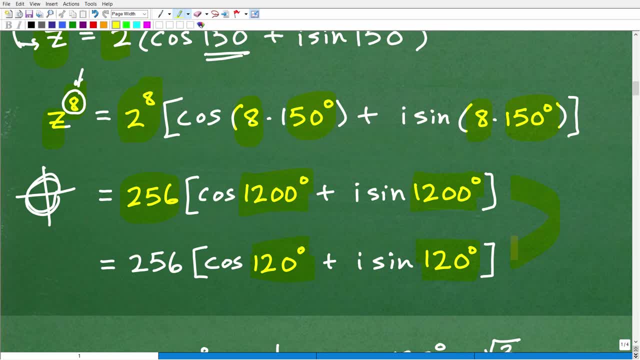 evaluate trigonometric angles okay, without the aid of a calculator. if you don't understand how to take a complex number and put it into trigonometric form, all those different things, you're not going to be able to handle DeMore's theorem problems. But anyways, 1200. 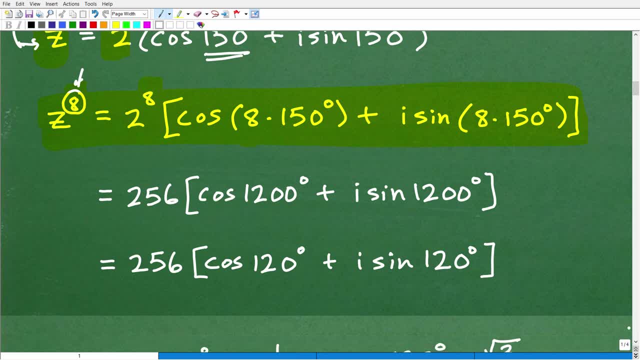 So again, you know it's a lot of work, All right. So, um, let's go ahead and do the actual um work here. Okay, The number crunching So two to the eighth is 256 cosine eight times 150 degrees. 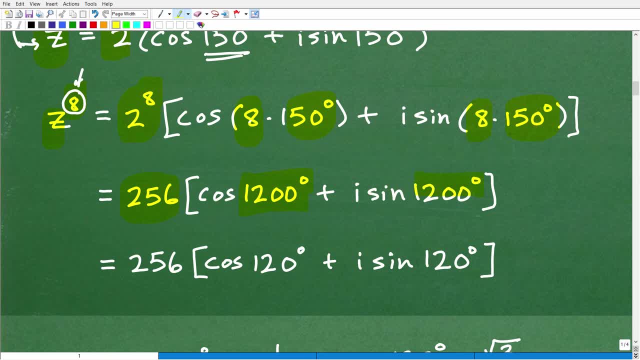 That's 1200 degrees. I sine eight times 150, 1200 degrees. Okay So 1200 degrees. If you uh looked at the unit circle, that's 360, that's 720.. It's going round, Robin. Uh, you would end up with. 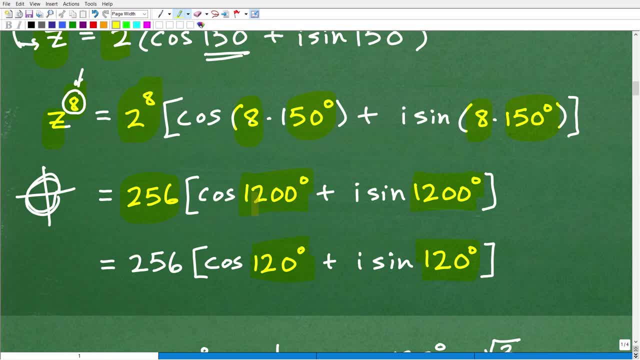 120 degrees as the reference angle, or 1200 degrees is the same as 120 degrees. This is how to evaluate trigonometric um angles. So again, DeMorse theorem requires your understanding. for a lot of things you've been studying in trigonometry. Okay, If you don't know how to. 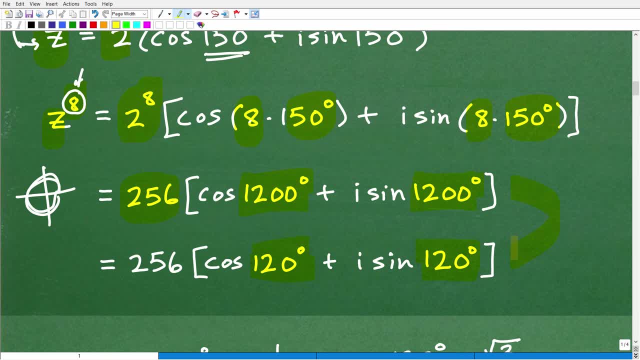 evaluate, uh, trigonometric, um, uh, angles, okay, Uh, without the aid of a calculator. if you don't understand how to take a complex number and put it into trigonometric form, all those different things, you're not going to be able to handle. DeMorse theorem: uh problems, But anyways. 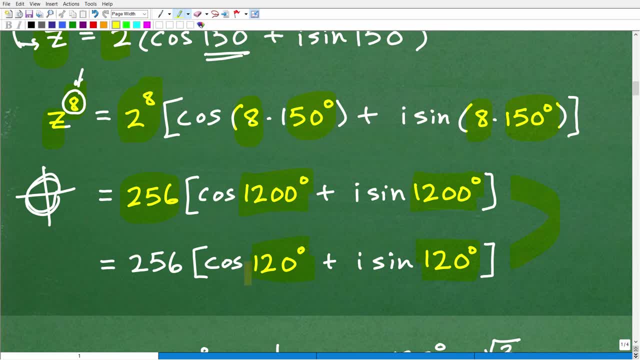 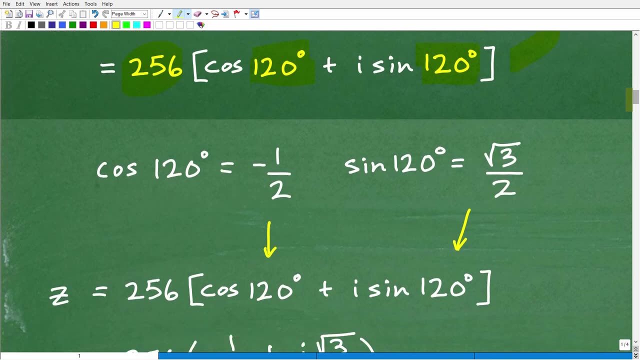 1200 degrees is if we, if we find the answer of cosine 120 degrees, it's equivalent of finding the answer of cosine 1200 degrees. So we have 256 times cosine 120, plus I assign 120 degrees. Okay, So moving on. So this right here was a bit of a of amount of work. So on cosine 120 degrees, 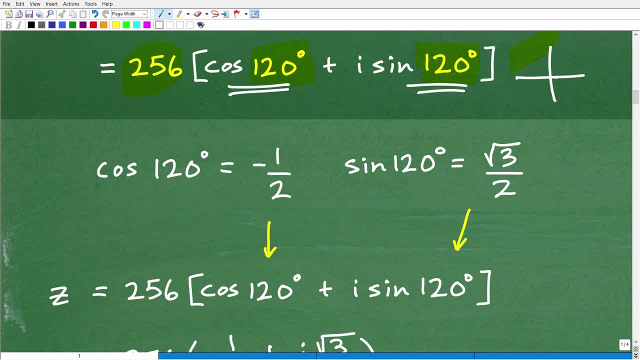 and sine 120 degrees. you're going to have to. you're going to have to. you're going to have to build a little reference triangle. Here is our initial side. You're going to have to figure out: uh, this is 90.. You're going to have to figure out the terminal side. You're going to have to. 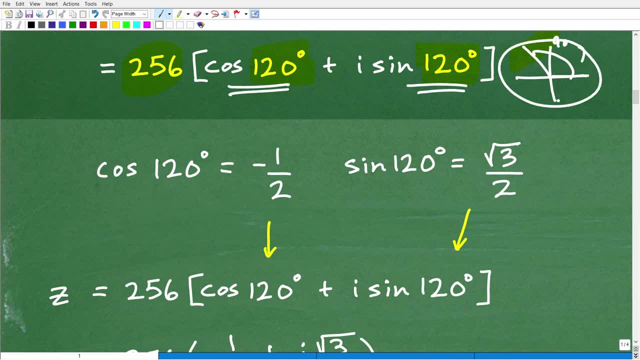 evaluate again this. if I try to teach you all of this, this video would go like 30 minutes And I'm trying to kind of uh focus on the DeMorse theorem application. So if you're a little, if you can't tell me with cosine 120 degrees and why it's equal to negative one, half right If you. 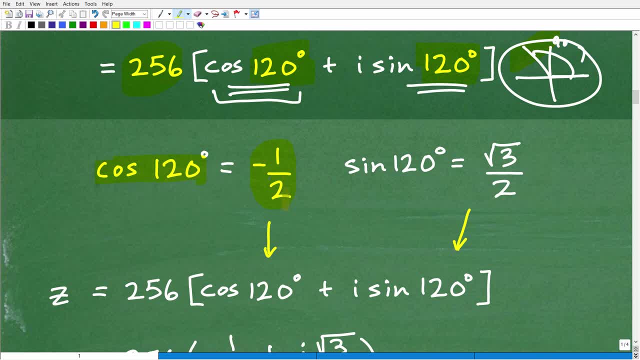 can't do this right here. cosine 120 degrees is equal to negative One half. then you're going to have to review that part of trigonometry, Okay. So, uh, when students struggle with DeMorse theorems, it could be all number. There's a lot of different reasons. 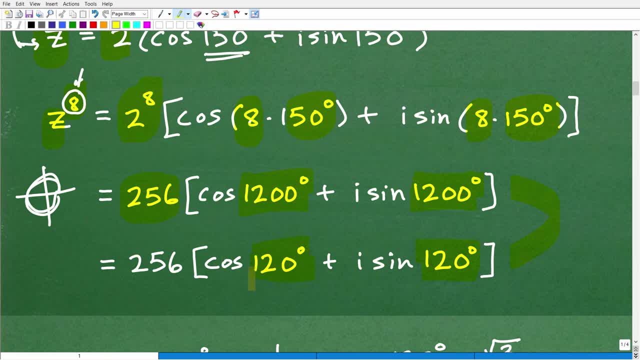 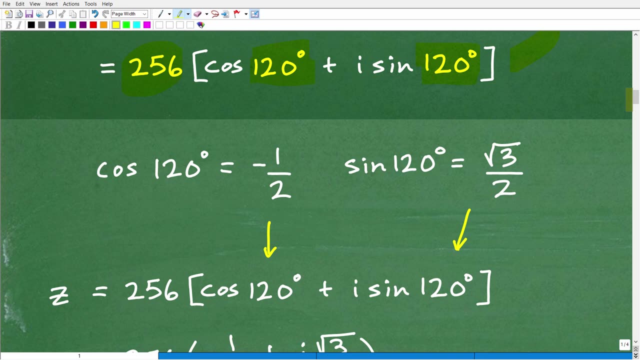 degrees is if we find the answer of cosine 120 degrees, it's equivalent of finding the answer of cosine 1200 degrees. So we have 256 times cosine 120 plus I sine 120 degrees. Okay, So moving on. So this right here was a bit of amount of work. So on cosine 120 degrees and sine 120 degrees. 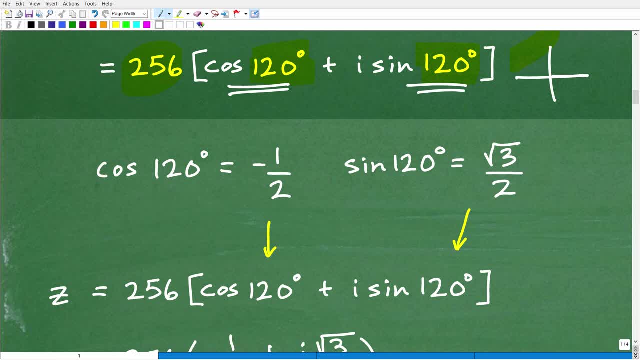 you're going to have to build a little reference triangle. Here is our initial side. You're going to have to figure out. this is 90.. You're going to have to figure out the terminal side. You're going to have to evaluate Again. if I try to teach you all of this, this video would go like: 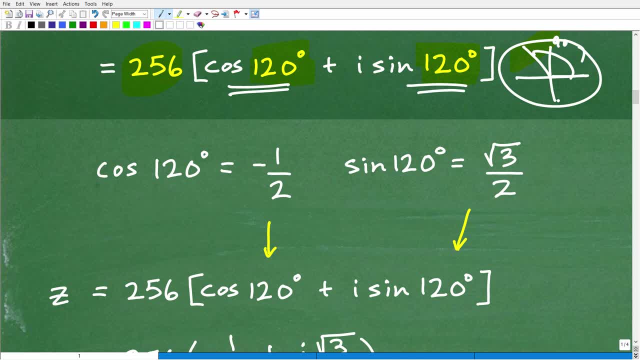 30 minutes. I'm trying to kind of focus on the DeMore's theorem application. So if you can't tell me, with cosine, 120 degrees and y, it's equal to negative one half, right? If you can't do this right here, cosine 120 degrees is equal to negative one half. So you're going to have to figure out. 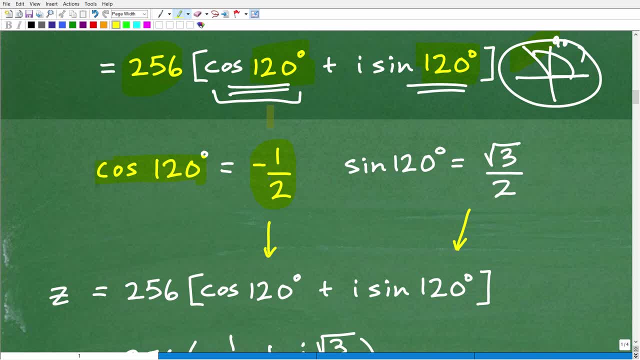 that part of trigonometry. Okay, So when students struggle with DeMore's theorems, it could be all number. There's a lot of different reasons why? Okay, Because you're using a lot of different skills here. All right. So cosine 120 degrees is equal to negative one half. Again, you're not. 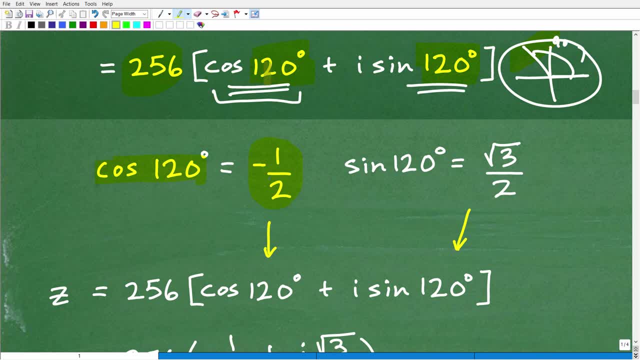 using your calculator for this particular problem. You could plug it in 120 degrees into your calculator and you'd get negative 0.5. But that you know you don't want to. you just don't want to do that. Okay, You want to see you can actually do that. So you're going to have to figure out. 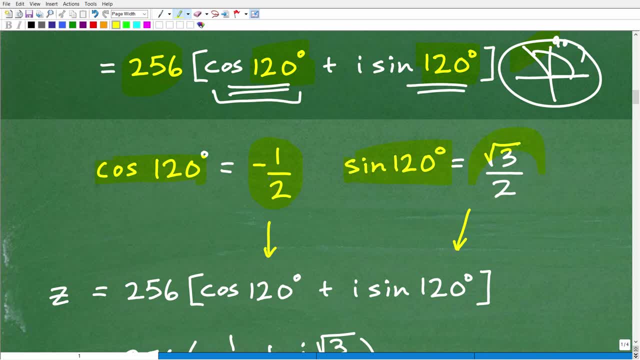 this without a calculator, All right. So sine 120 degrees is square root of 3 over 2.. Okay, So here we just figured out what cosine 120 degrees is and sine 120 degrees is. So we're going to go ahead and plug in and substitute these values in for those values, And this is what we got. 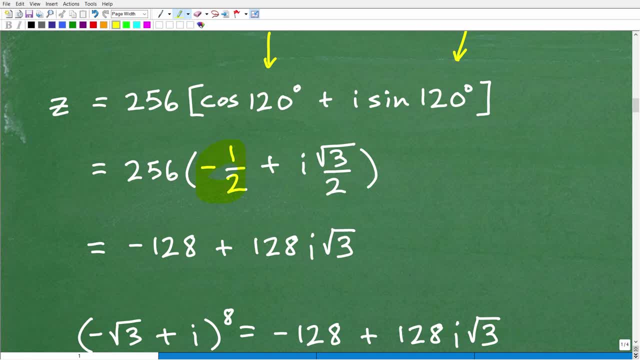 All right, So again, 256 cosine 120 degrees, that's a negative one. half Sine 120 degrees, that's square root of 3 over 2.. So I have 256 times this. I'm just going to go ahead and. 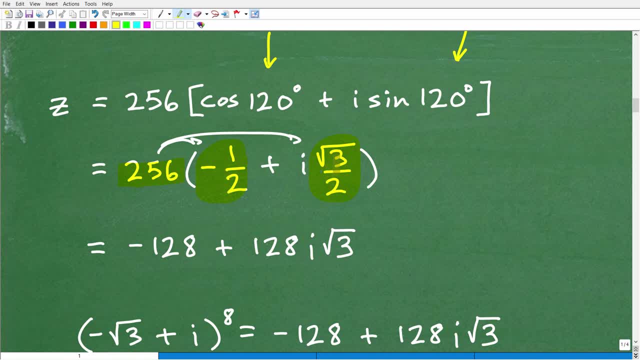 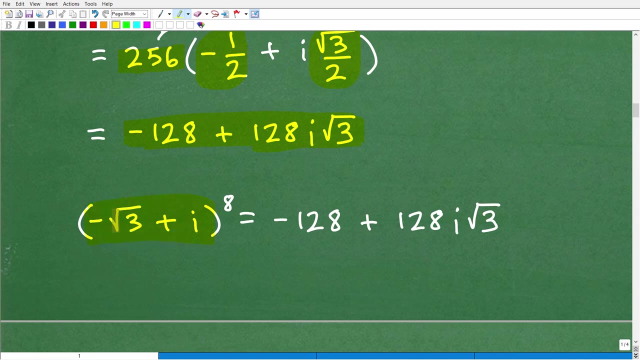 distribute that 256 into negative one half and square root of 3 over 2 times i And you get negative 128 plus 128 i square root of 3.. That is the answer. Okay, So let's just kind of come full circle. Our original problem was the square root of 3 plus i to the eighth power. Okay, This. 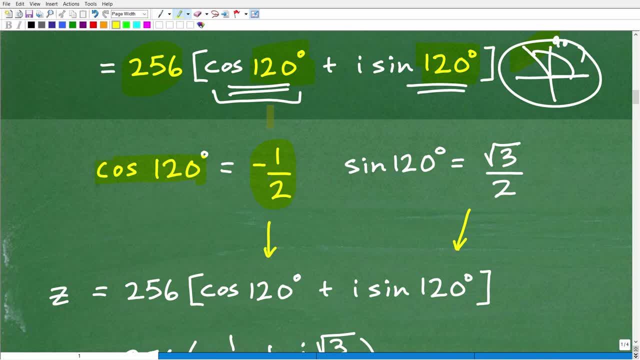 why? Okay, Because you're. you're using a lot of different skills here. All right, So uh cosine 120 degrees is equal to negative one half. Again, you're not using your calculator for this particular problem. You could plug it in uh 120 degrees into your calculator and you'd get. 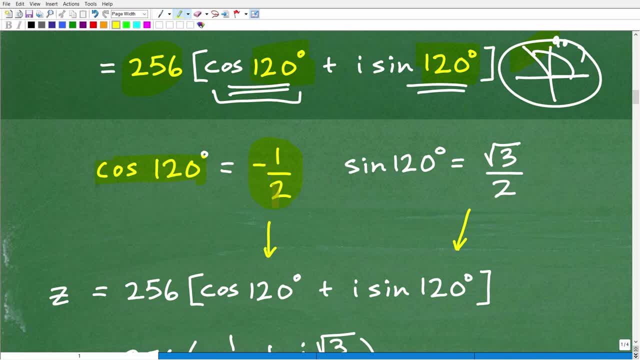 negative 0.5, but that you know. you don't want to. you just don't want to do that. Okay, You want to actually do this without a calculator? All right. So sine 120 degrees is square root of three. 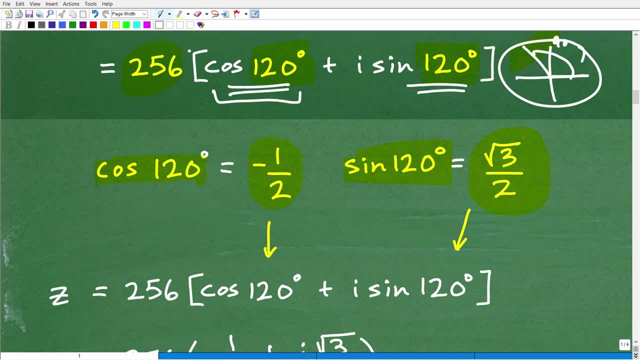 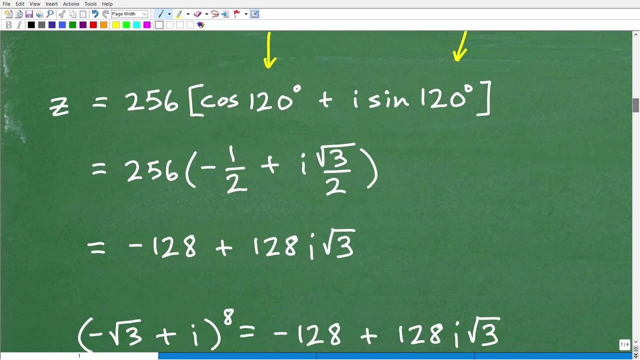 over two. Okay, So here we just figured out what cosine 120 degrees is and sine 120 degrees is. So we're going to go ahead and plug in and substitute, uh, these values in for those values And this is what we got, All right. So again, 256 cosine 120 degrees. that's a negative. 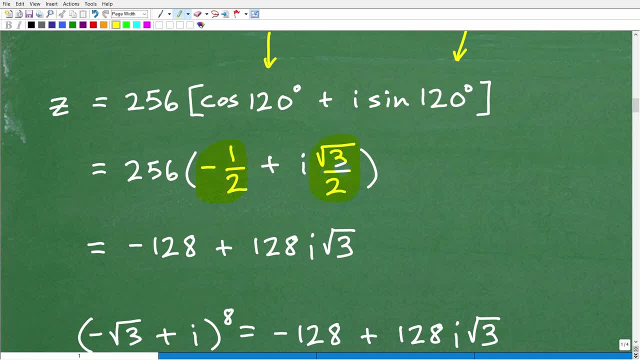 one half uh sine 120 degrees. that's square root of three over two. So I have 256 times this. I'm just going to go ahead and distribute that 256, uh into negative one half and square root of three over two times I and you get negative 128 plus 128, I square root. 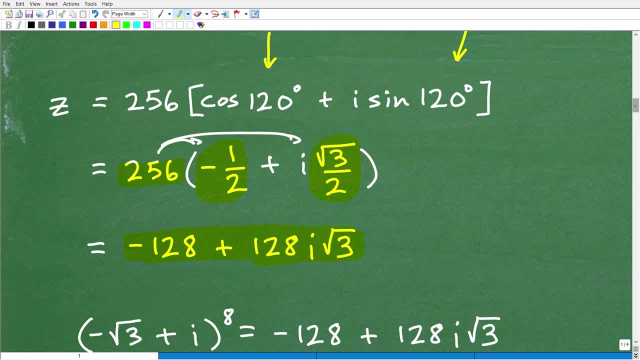 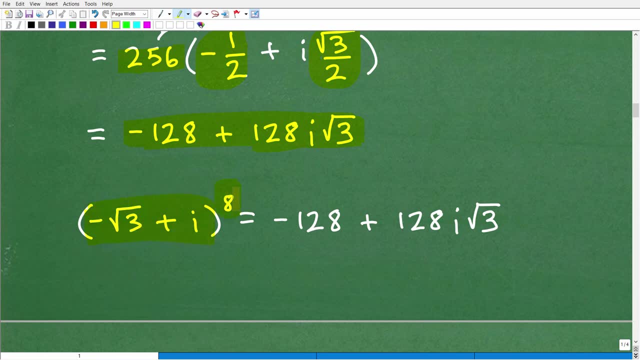 of three. That is the answer. Okay, So let's just kind of come full circle. Our original problem was the square root of three plus I to the eighth power. Okay, This is our complex number: A plus B I form. We're taking that to the eighth power, And here our answer is in: A plus B, um I form in. 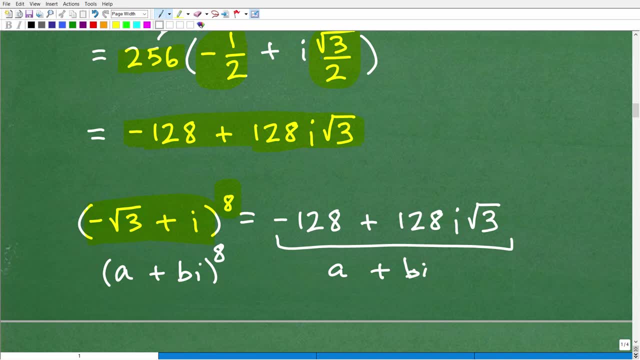 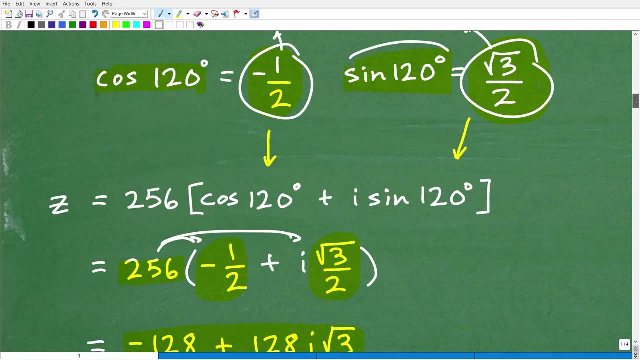 rectangular form. Now, if your teacher was really mean, they could say: take, you know, find the answer. and trigonometric form, Okay. And you'd be like, Oh no, I'm going to have to go backwards. No, no, you actually had it right up here, Okay. So this is the answer in a trigonometric form. 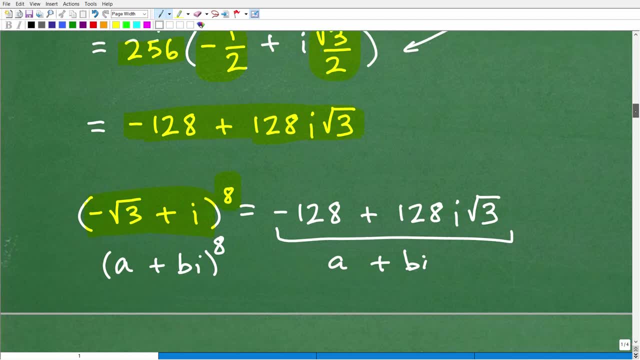 but we put it back in to rectangular form. So you're going to be asked all different sort of aspects And you know like you've got to be very, very careful on what your teacher's asking. Um, sometimes they'll give you their complex number. 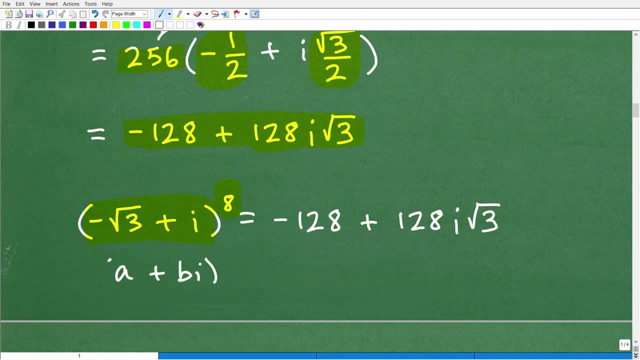 is our complex number a plus b, i in Rectangular form. We're taking that to the eighth power And here our answer is in a plus b i form in rectangular form. Now if your teacher was really mean, they could say: take, you know. 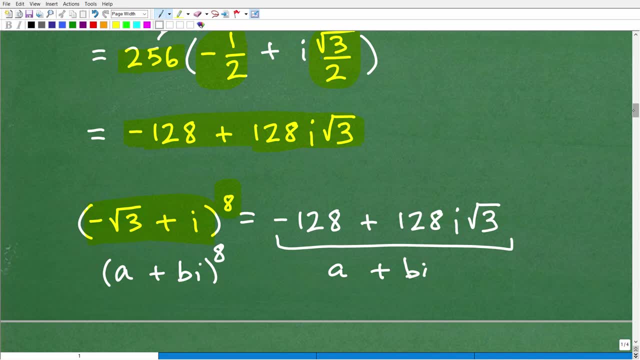 find the answer in trigonometric form, Okay, And you'll be like: oh no, I'm going to have to go backwards. No, no, you actually had it right up here. Okay, So this is the answer in trigonometric. 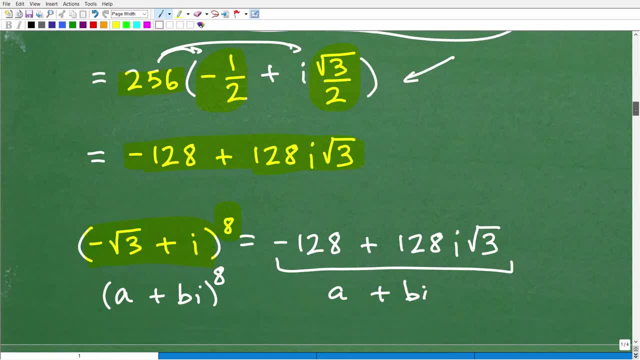 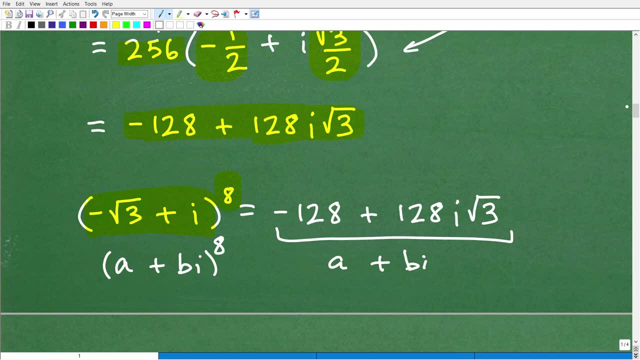 form but we put it back in to rectangular form. So you're going to be asked all different sort of aspects And you know like you got to be very, very careful on what your teacher's asking. Sometimes they'll give you their complex number already in trigonometric form, but more often than 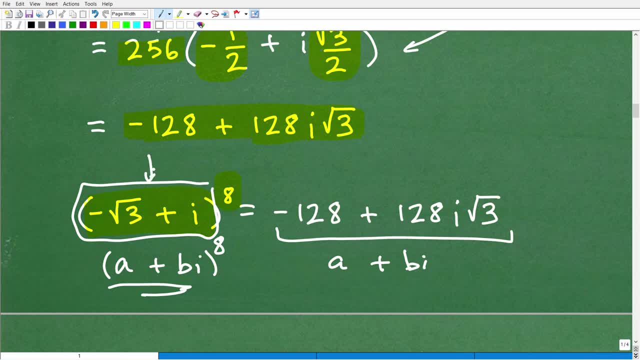 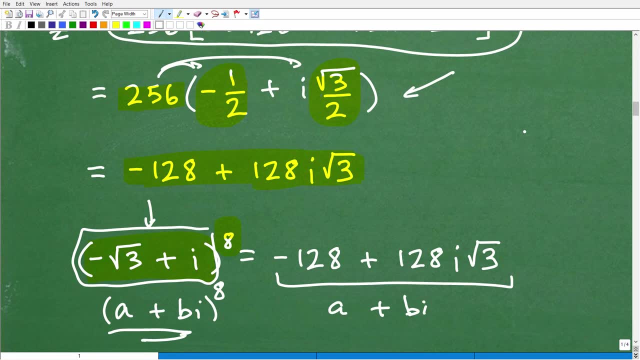 not, you're going to get it in rectangular form, You're going to have to put that into trigonometric form and then you're going to go ahead and apply demorphs there. Now, if you got this problem right, then I must give you an awesome, happy face with a good old 1985 Mohawk. 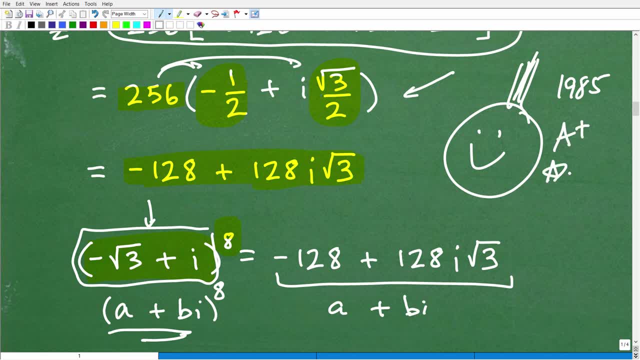 with extra Aquanet hairspray a plus. I'm going to give you several stars because this is a lot of stuff and 100% You know you're doing really, really good. If you're able to do this, then you're definitely on the right track, And 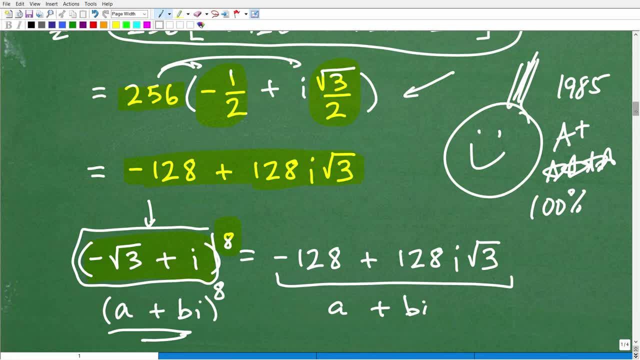 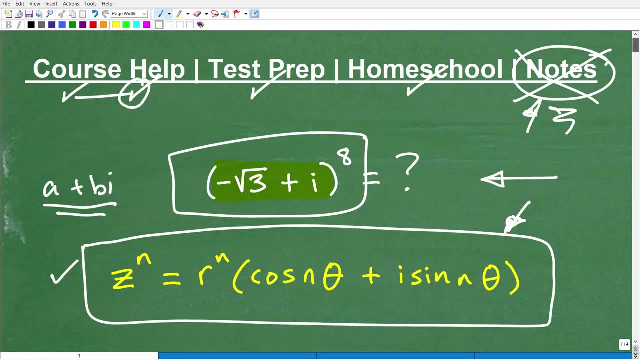 you're showing me that you know a lot of subskills in trigonometry. Okay, So demorphs theorem is one of these type of topics in pre-calculus that you have to use a lot of the things that you've already been learning, So, but anyways, we got this right Excellent. 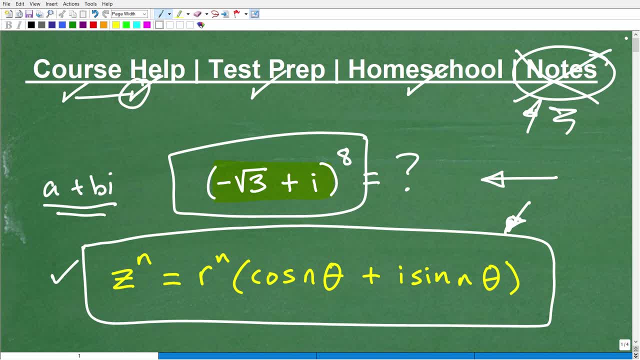 If you kind of like understand demorphs theorem a little bit better from from this, then that's the whole idea of this video And if that is the case, please consider smashing that like button If you watch this video and you're still lost. listen, I get that as well. 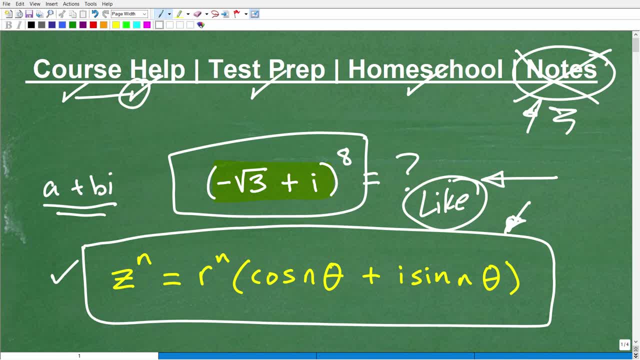 You're going to need additional help. I don't have. I don't think I have too many videos in my pre-calculus playlist on my YouTube channel, but I do have some things in there that can help you out. I would strongly recommend you checking out my pre-calculus course to really you know.